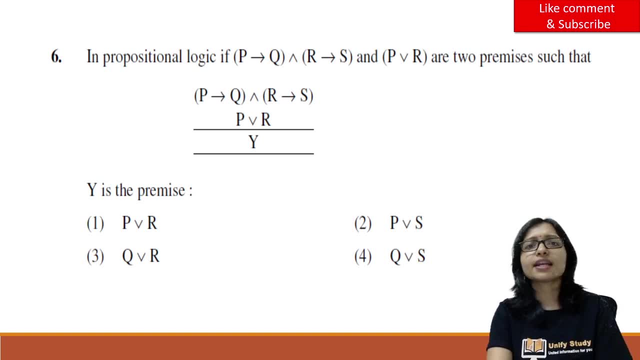 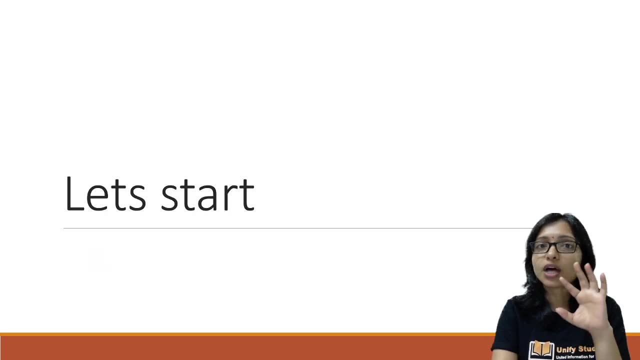 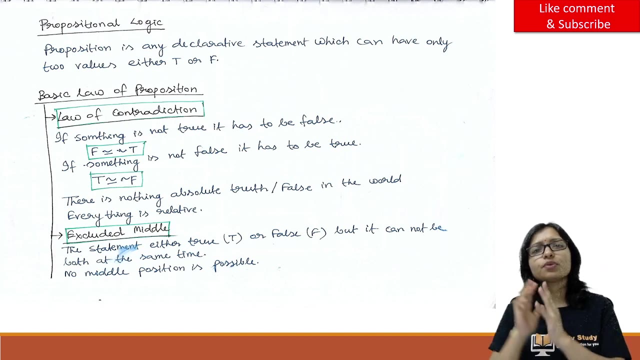 wrong. Someone will tell you this is correct answer, but you are getting confused Why this is correct, Why this is wrong, Right, So that's why, in this video, I will tell you the total understanding, from basic to advanced level, all the basic concept. with that we will solve these. 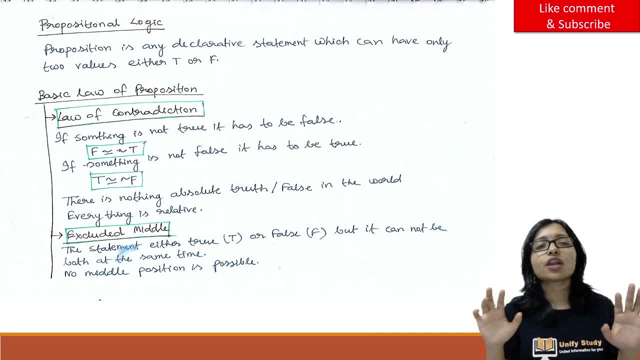 all question and after watching that, your total concept will be clear from proportional logic And predicate logic, because proportional logic and predicate logic is a very important area from where so many questions are coming. Whatever exam you are preparing, if it is your college exam- 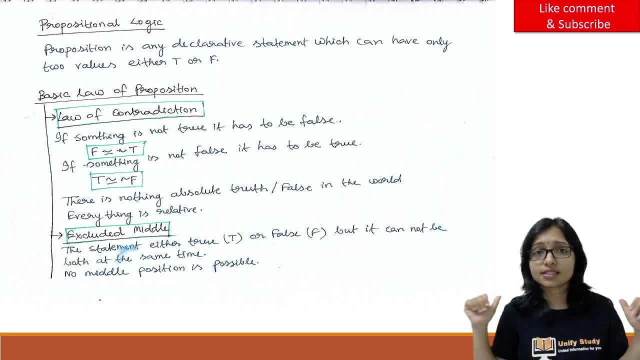 UGC net exam, gate exam, any other competitive exam in discrete math. this is a very important subject and it is related to artificial intelligency also. That's why you cannot leave it. So let's start. Must watch till the end. Don't leave in the middle. Don't leave till the end, Don't. 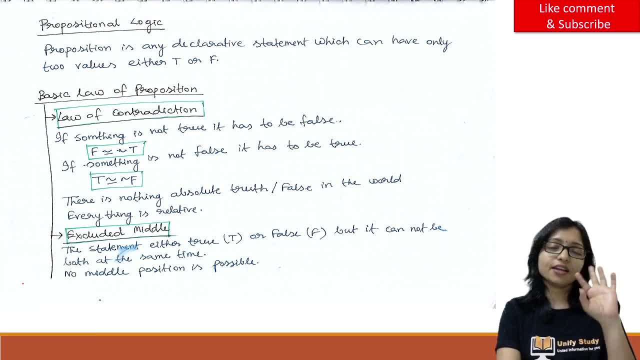 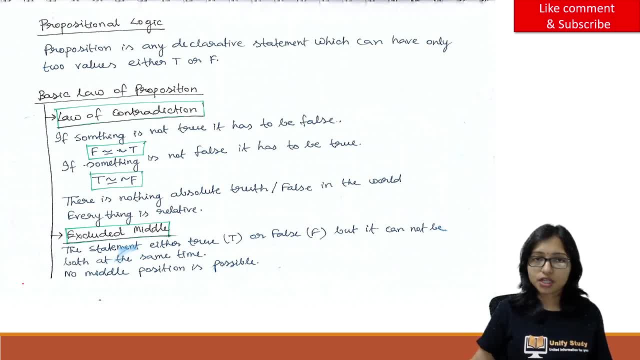 see in the proportional logic. first of all, what is proportional logic? Proportional logic is working with true and false. Yes, there is no middle. How are you? I am good or bad. There will be no answer like that. I am so. so It's going on. No, Either yes or no. Either yes or no. Either yes or 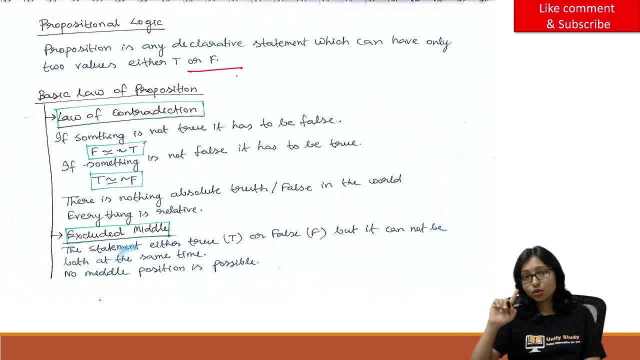 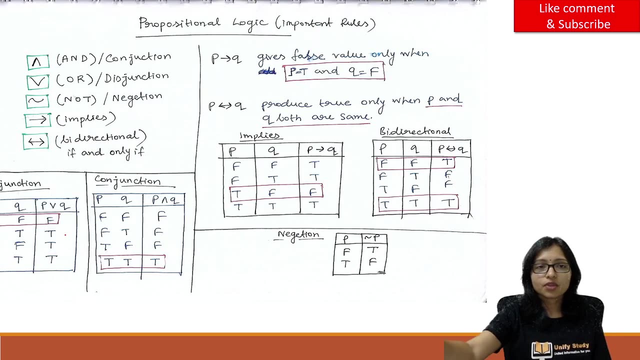 false. Either true or false. There will be no in between. result: This is proportional logic. So excluded middle means in between, anything will be not there. Not false means true, Not true means false. And here are some table we have to remember, And these are the table actually just related with: 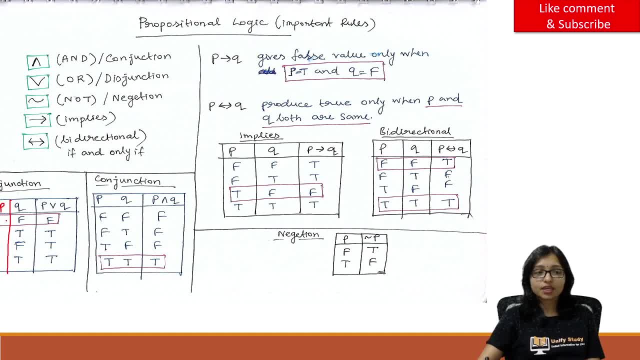 the digital logic also. Same thing are here 0, 0,, 0,, 1,, 1, 0, and 1, 1.. That is the or You did the or right. That is called disjunction Or means. 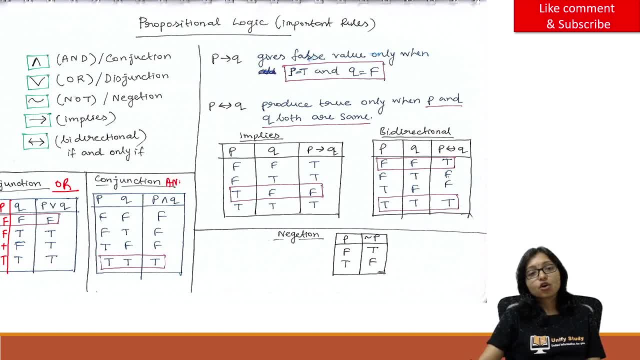 disjunction And means conjunction, And we did that. P, Q and This is the and table. How this is working In the or table. when there was or table for P and Q, then there is or 0, 0,, it will be 0.. 0, 1,, 1.. 1,, 0, 1.. And 1, 1 will be also 1.. That is the or That is actually. we are writing in this way. This is the symbol of or in propositional logic. 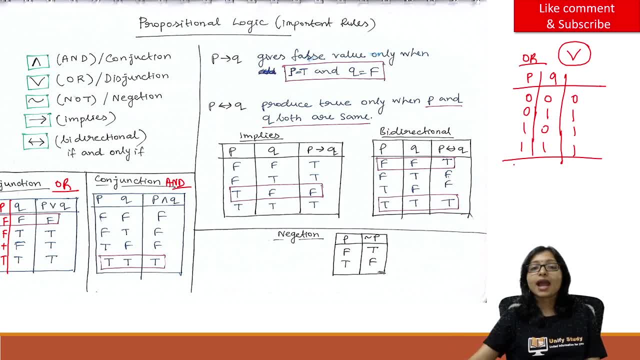 Predicate law In here, the what is and And is how we are writing. and Same way, 0,, 0 is 0. In and when both are 1, then only it is 1.. That's why that is true. 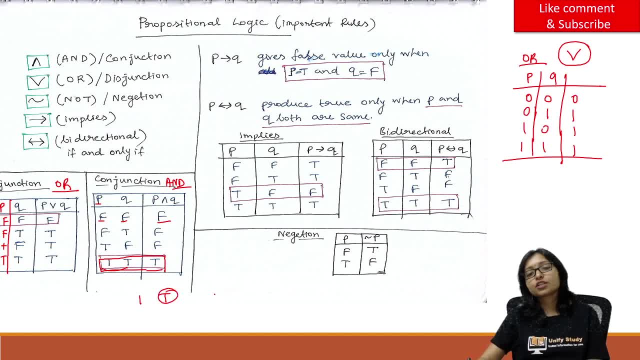 Instead of 1, we will write here true And instead of 0, we will write here false. Actually, propositional logic, if you are learning through digital logic concept And sometimes the problem can be solved, Most of the time the problem can be solved in digital logic format. also Because propositional logic, this type of symbol it's getting, we are getting confused. What is this? What is that? Other than that, if I am writing this one like this way: P bar plus Q. 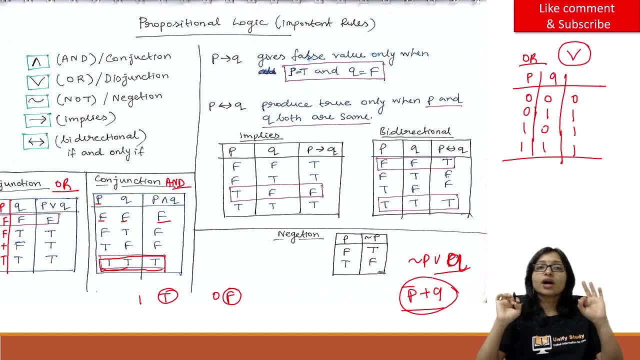 then we are feeling so happy, right. So this is one trick: Whenever you saw the proportional logic question, just change it into digital logic format, Like Boolean algebra. we will solve it. It is very easy for us. So here is something extra also, what is not there in digital logic. 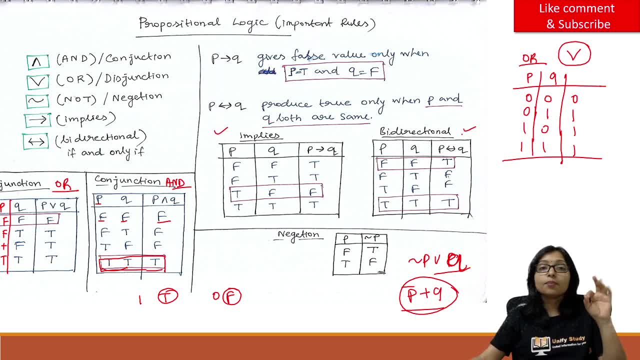 That is the implication and the bi-directional Implication means P implies Q Means if P is true, then Q is true, Like that type Means if, then when we are telling if, then then we will apply the implication symbol. What is then double implication? Double implication is like if. 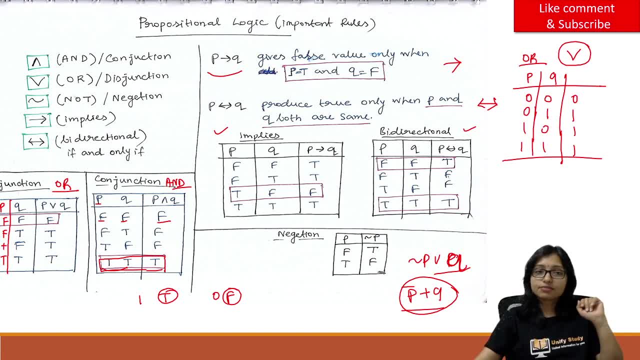 and only if. Because when I am telling that if today is Monday, then I will take the class, It does not mean that I am taking class means it is Monday. It can be any other day also. So here is another trick: If today is Monday, then I will take the class. 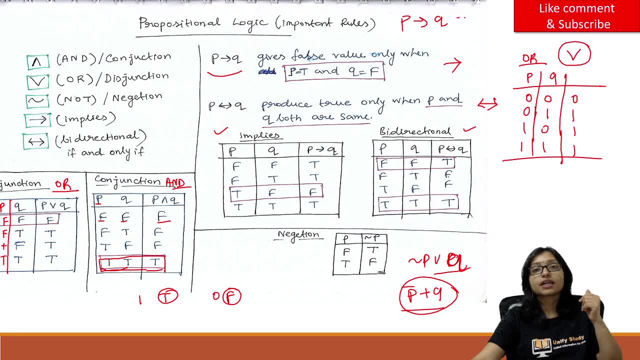 Here the problem is: if I am telling P implies Q, that does not mean Q implies P also. But in double direction means when we are telling bi-directional, double implication, then it is actually: if P equals to P implies Q and Q implies P, both are correct. That's why, if and 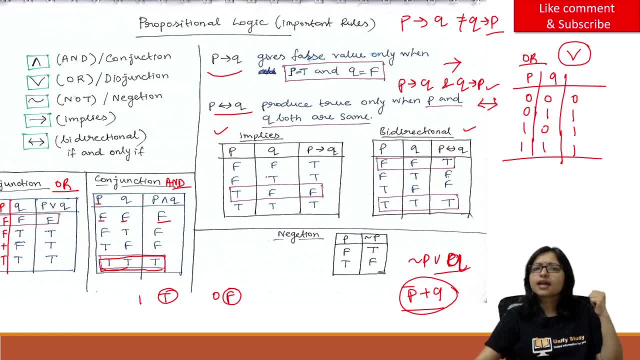 only if. What is the truth trouble here? Here the truth trouble is very interesting. You can see: when both are false Means P is also false, then Q is also false. If today is not Monday, I will not take the class. 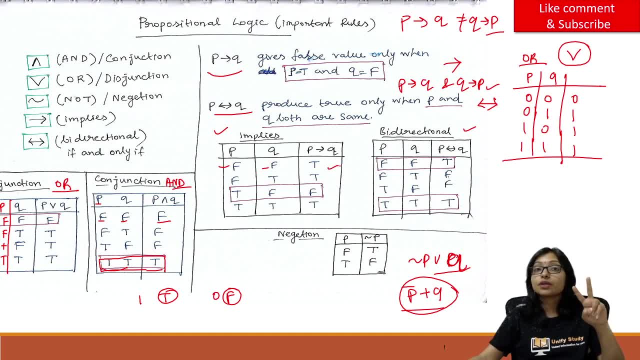 So both are false. That's why P implies Q will be true Here. if P is false but Q is true, It can be happen. It's not Monday, but I am taking the class. It is another weekday- Tuesday, Thursday. 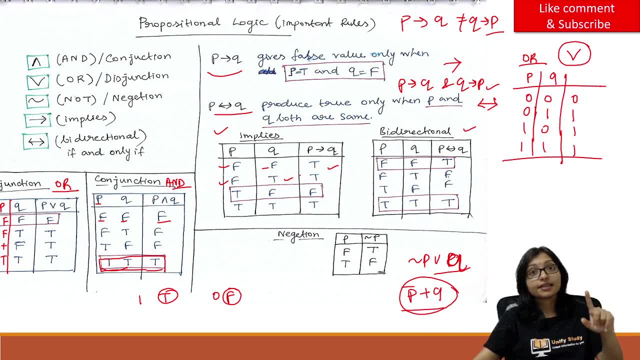 Friday, It can be any day. I am taking the class. Yes, So when P is false, Q can be true. That's why it is also true: P implies Q. Now, P is true. It is Monday. I am not taking class. It is. 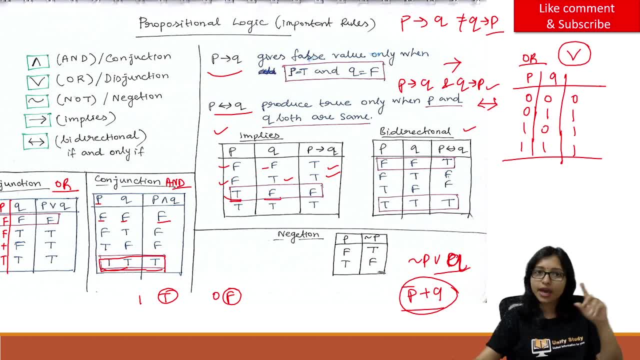 false. Normally it will be false because P is true here, So you have to take the class right. So that's why it is false, True, true, though always true When both are true: the P it is. 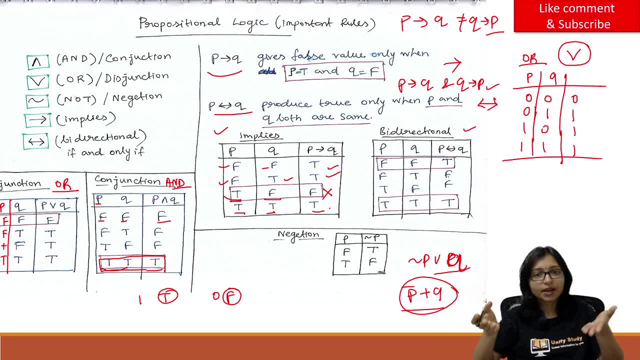 Monday I am taking the class: Implies is true here, It implies, implication is true here. So this is the truth. trouble for the implication. What is the truth? trouble for bidirectional. Bidirectional means both have to be same. That's why, for false, false it will be true, and true, true also, it will be true. 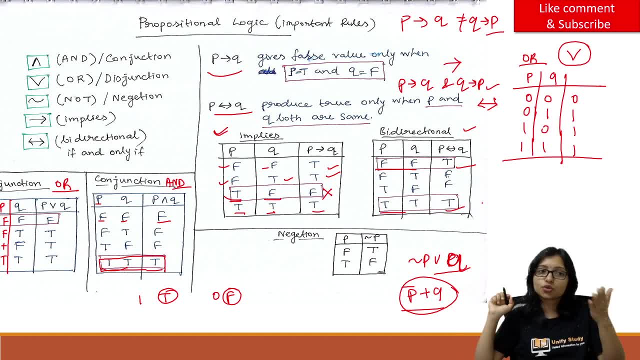 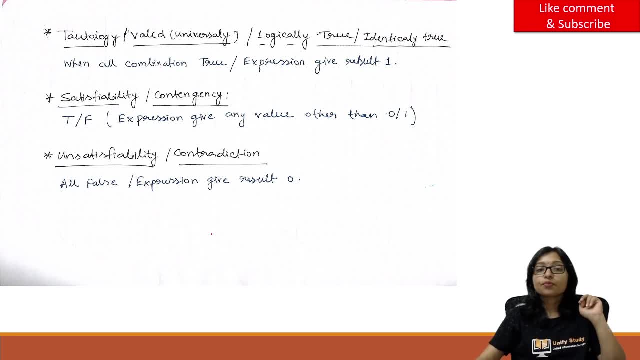 These are the main truth, trouble, what you have to remember. So it is and or implication, and bidirectional. Now here is another next important thing, that is: P implies. Q means what P implies. Q means not P or Q. This is a five star formula. from where means always. you have to apply this formula for solving 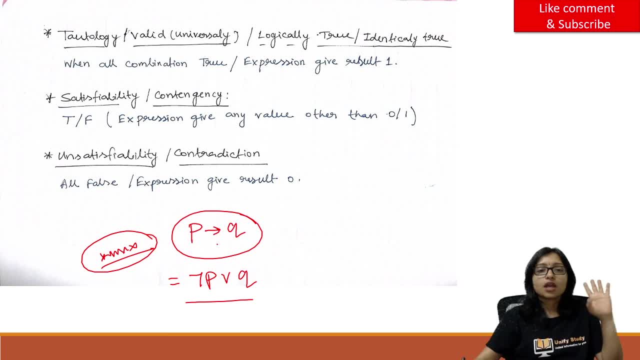 proportional logic, predicate logic. everywhere P implies Q is not P or Q. This is, please stick in on your mind, everywhere it will be required. Now the next type of question are coming, what is called tautology: valid, identically, true, satisfactory. 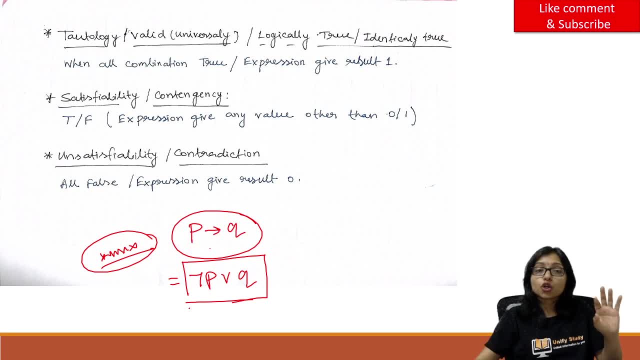 What is that? I am telling you? simply tautology, or valid, or logically true, or identically true. these all are same. When it is, when all the combination is true- all combination true means any expression will be given to you, like maybe P or Q and P bar, like something. Then if I am telling, 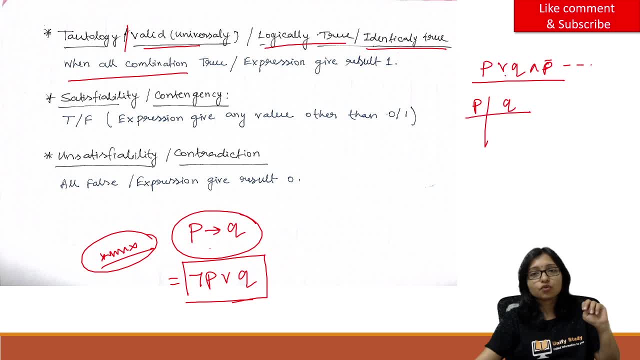 this two truth trouble: P, Q, The two variable. using this variable, if I am putting in this expression, if for all combination I am getting true result, all the combination I am getting true result means it is true. Otherwise, another way also we can solve just by solving the expression. If I am solving the expression P plus, 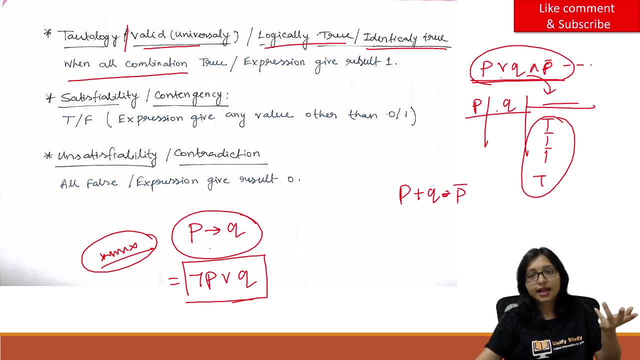 Q, dot P bar. it is like that, After solving, if I am getting expression giving result one, then it will be true, otherwise it will be false means, then it will be tautology or valid. What is then? satisfiability or contingency? 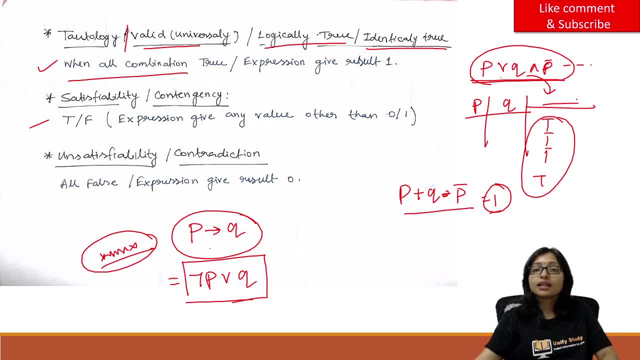 Satisfiability or contingency means, when you are solving this expression, if you are getting in the truth trouble. Some of them are true, some of them are faults. like this way, combination of true and false, then that is called satisfiability or false. 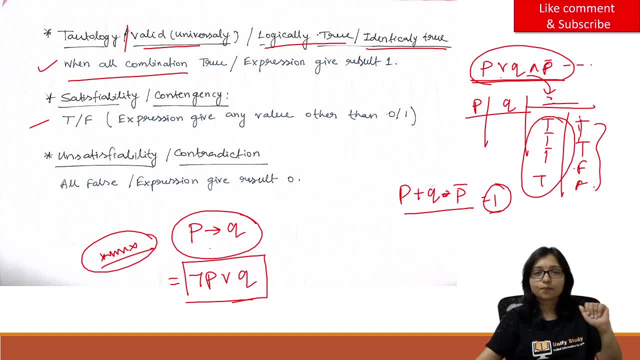 called satisfiability or contingency. When you are solving the expression, you will get a value in a terms of variable Expression. give any value other than 0 or 1 in a terms of variable, like either p, p, bar, q or pq or something. It will be not 0 or not 1.. It will be in a terms of variable. 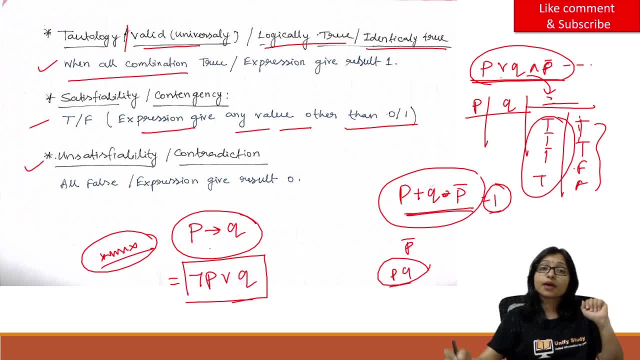 then it is satisfiable. What is unsatisfiability then? Unsatisfiability or contradiction means when expression gives result 0 after solving how it is p dot, p bar, but the expression will give you 0. So when you are getting expression result 0, then that is called contradiction. This is 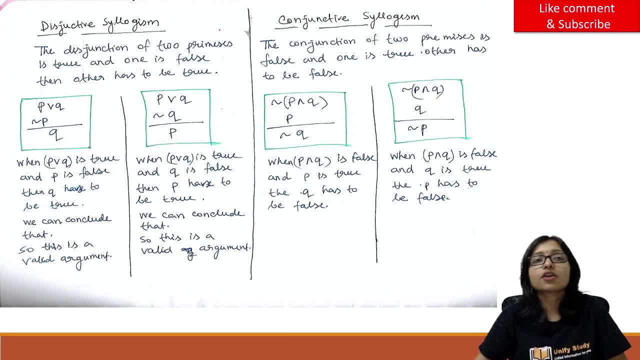 simple. Now think here there are called the disjunctive syllables, Syllabism and conjunctive syllabism. What is that Disjunctive syllabism? it is the format of syllabism. What is the format Here actually? whatever given in the upper side, In the upper. 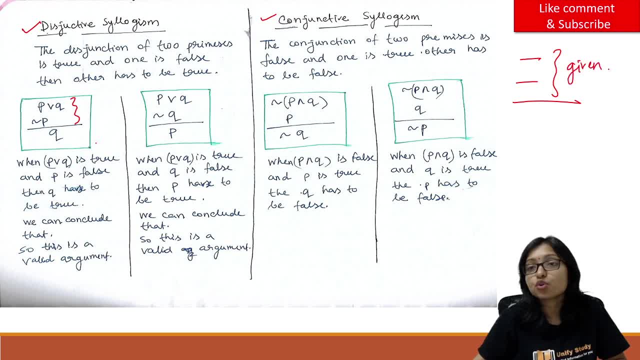 side there are two statement will be. these are given true and in the lower side it is the conclusion. you have to prove that from the given true is it coming true also always? If it is the conclusion coming true always, then we can solve it. So this is the format of syllabism. 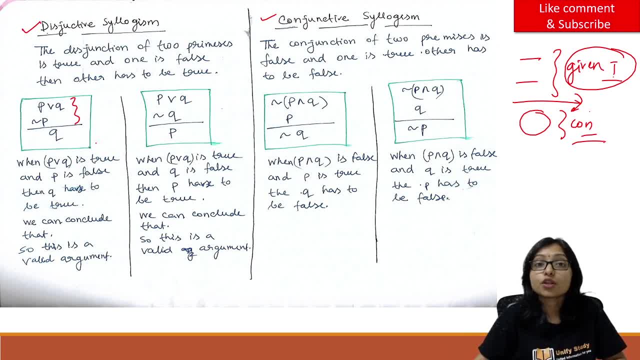 We can say it is valid. Otherwise it will be not valid. So you can see here what is going on. p or q is, given true Means, what it is Actually. p plus q equals to 1. p plus p or q, given true means it is. 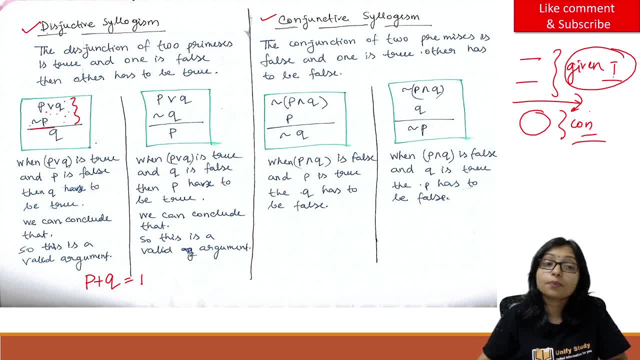 1.. Another one is also given. that is not p is true. So what is another one Not? p equals to 1.. So what is p? p equals to 0.. So if I put here, 0 plus q equals to 1.. So what is the value of q? Definitely? 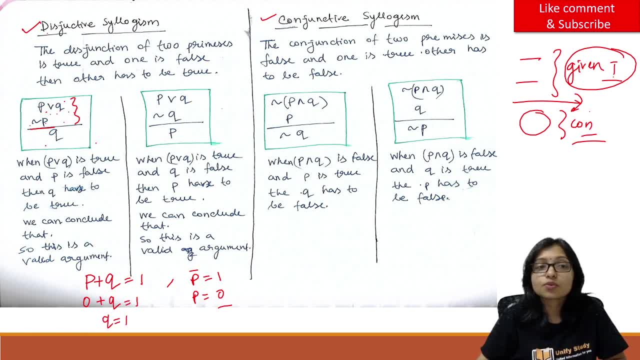 the value of q is 1.. Right, So that is why q is true. Yes, the conclusion is correct here, And that is why it is a valid one. Same way is there. that is, p plus q equals to 1, given not q is 1. 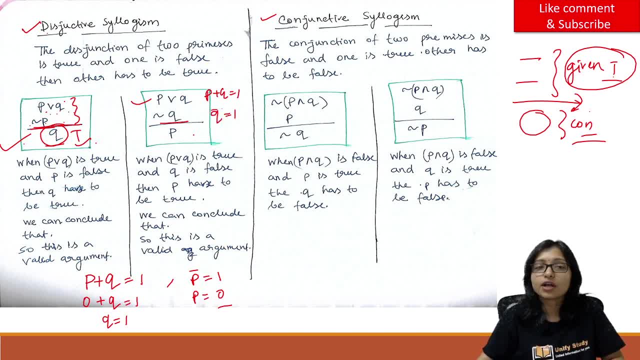 given means q bar is 1, given q equals to 0. So p will be 1.. And when I am doing conjunctive syllabism, what is conjunctive? It is given that p dot q bar equals to 1.. p dot q complement means bar equals to 1.. Right, And here the p equals to 1.. So when p equals, 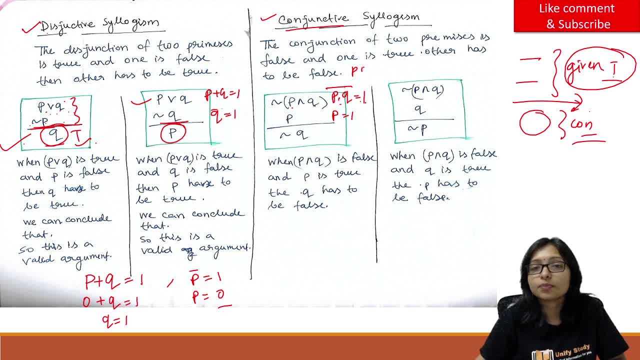 to 1 and its bar equals to 1. means what, Actually? p, q equals to 0. So why it will be 0?? Then q bar is true means q bar is true. So when p equals to 1, it is given that p dot, q bar equals to 1.. So 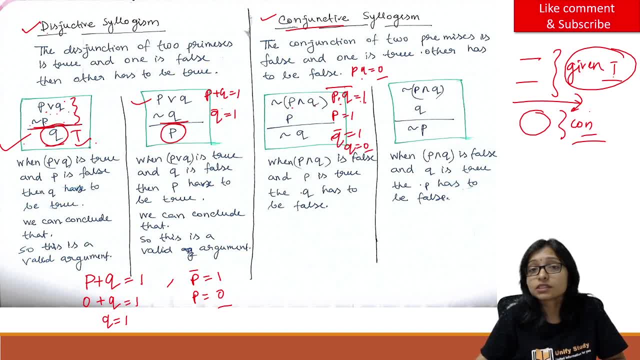 bar is 1 means q equals to 0. So q equals to 0. that is why p q equals to 0.. This is the conjunctive syllabism. Something is given to you from the given thing. am I getting the conclusion? 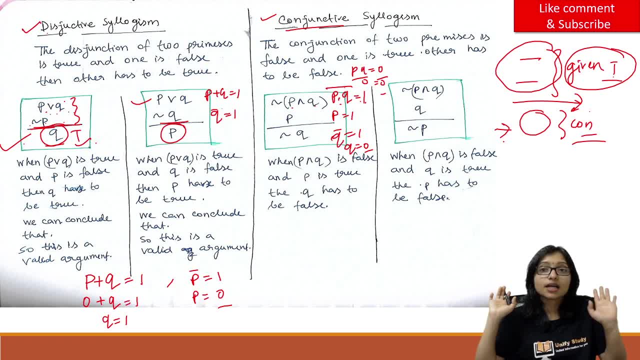 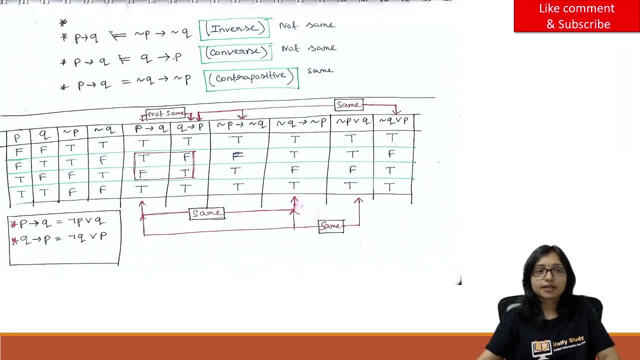 If I am getting the conclusion, then that is called the syllabism is valid here. This is the format. Now we are going to another thing that these are also three important, most important: P implies q equals to 0, p implies 0, q. It is inverse, It is not same. It is not same When I 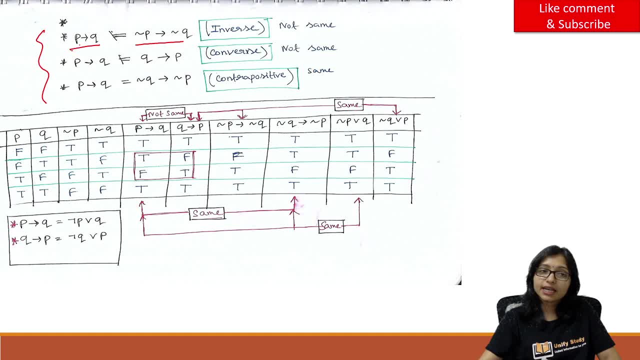 am adding inverse. that is not same, That I am telling that if it is Monday I will take the class. Not Monday I am not taking class. No, it can be true It is not Monday, but still I can take the class. So inverse is not same. P implies q. I cannot say q implies p. This is called converse. 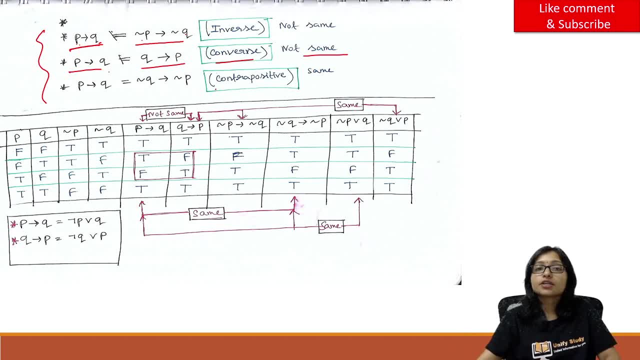 This is also not same, But the contrapositive it is same. P implies q equals to 0, q implies 0 p. that is same How this is coming. P implies q means I can write 0 p or q I can write it. 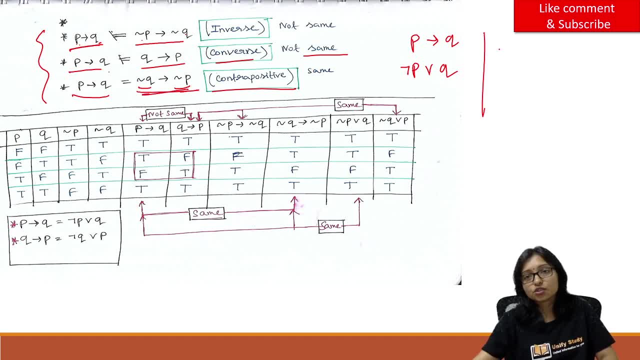 Now, here you can see if I am doing this. one 0 q implies 0 p. What it will be: 0 0 q, because p implies q is negation. So 0, 0 q or 0 q. 0 p means it is 0 0 q or 0 p. 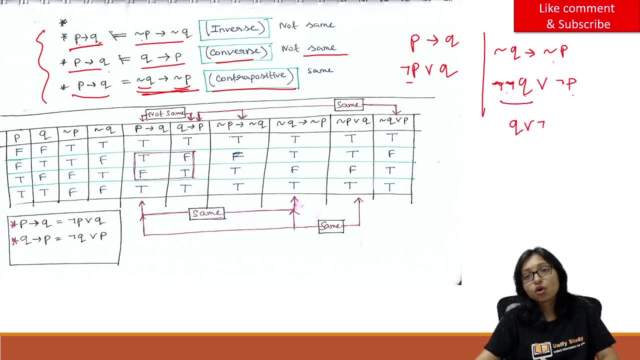 So double negation means what That is: q or 0 p? Now, same thing. I can write like this, because: or see that here, if I am writing q plus p bar, that is same. I can write p bar plus q, Right. So that is why I can write here: 0 p or q, So it is same. 0 p or q, 0 p or q, It is 0 p. 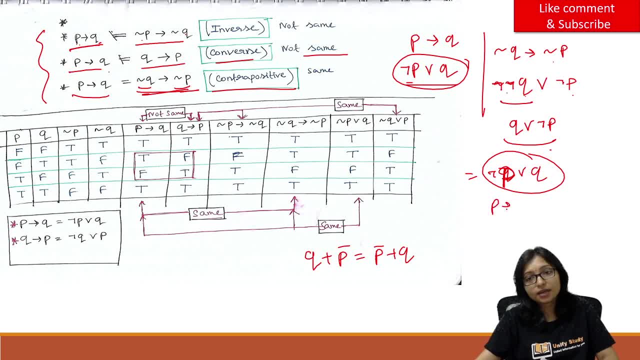 0, p or q, It is same Means it is actually p implies q. So that is why p implies q equals to 0, q implies 0 p. This, this formula. that is why every time you will apply this formula, And double negation means the same value, Double negation means it will come to the same. 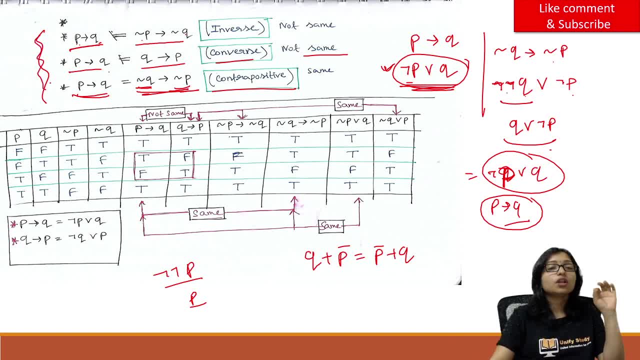 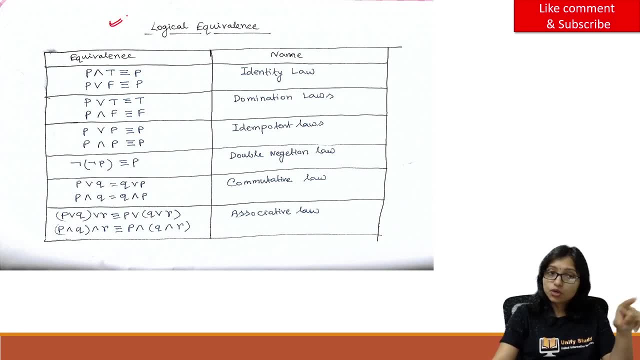 So this is a very important, Always remember this- three rule in proportional logic, And these are the rule of logical equivalence. That rule is same as the rule of the digital logic. In digital logic you learn that p dot 1 equals to p Right And p dot 0 equals to 0. Even, also, you learn that p plus 0 equals to p. 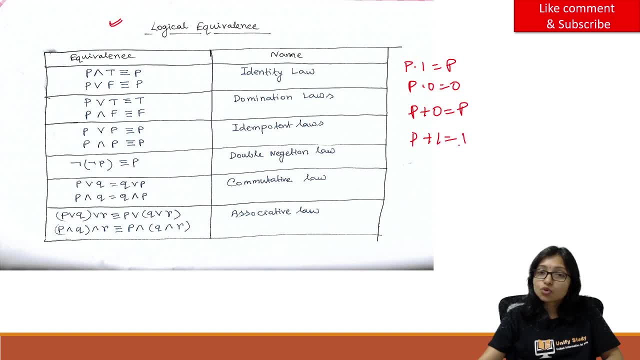 And p plus 1 equals to 1.. Anything plus 1 is 1.. Right, So that these are the identity law, dominance law, You know that. And idempotent law means when I am doing p dot, p that is p, P plus p, that is also p. These are the law. 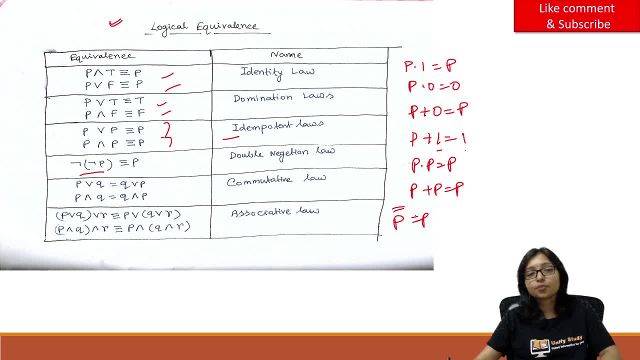 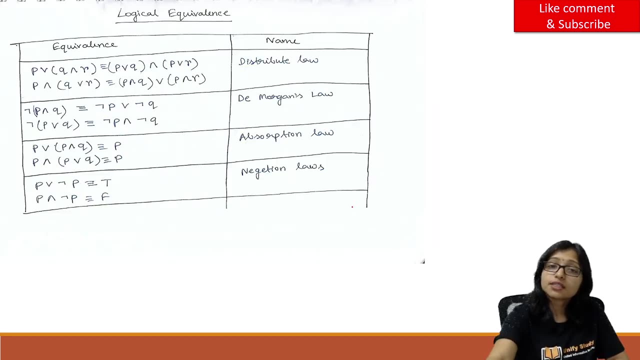 Double negation: p double bar equals to p. Commutative law. also, you know associative law means what p Plus q plus r. I can write p plus q plus r. That is the associative law. Same thing, Digital logic. Think like a digital logic way. 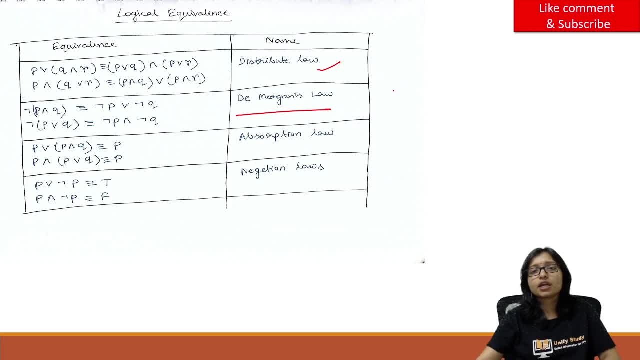 Distributive law and de Morgan's law is very, very important In digital logic also, In proportional logic also. So when you are doing p q bar, then it will be what p bar plus q bar, And when I am doing p Plus q whole bar, then it will be p bar dot q bar Right. This de Morgan's law is the next, another one where it will be required for always simplification. 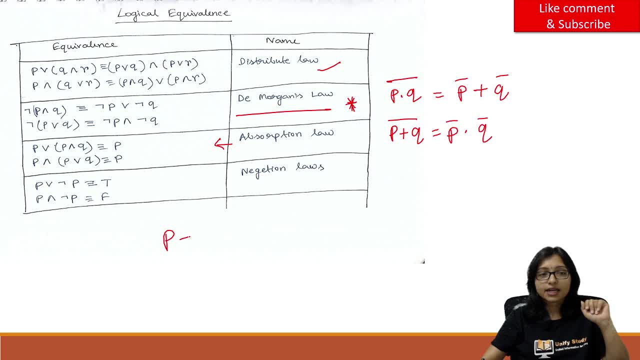 And the absorption law is also very important. when I am writing p plus p q, then it is actually p P plus p q. If I am doing p dot p plus q, then also it is p P plus p q and p dot p q. These are absorption law. So p plus p q will be p only and p dot p plus q also will be p only. 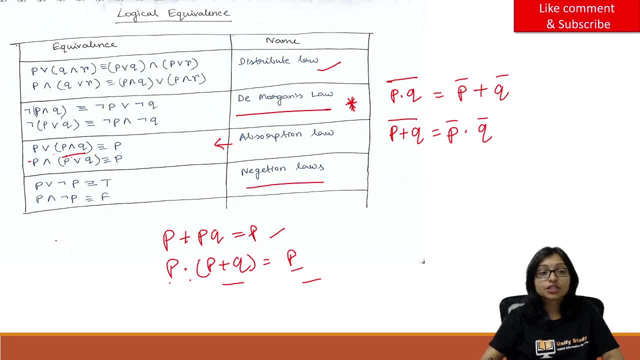 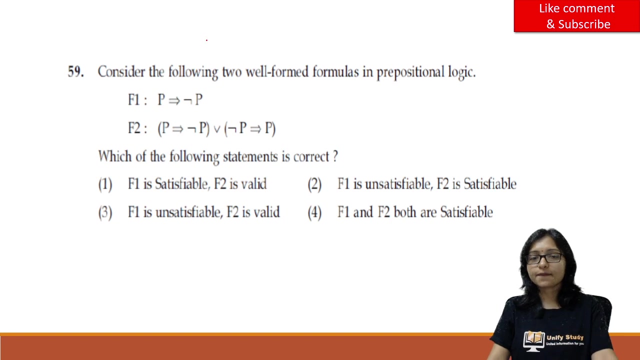 These are the some very, very important. and another one negation: that is, p plus p bar equals to 1 and p dot p bar equals to 0.. So these are the simplified rule, simplification rule, what you have to apply for digital logic. And now I'm going to talk about how to solve the question, one by one. 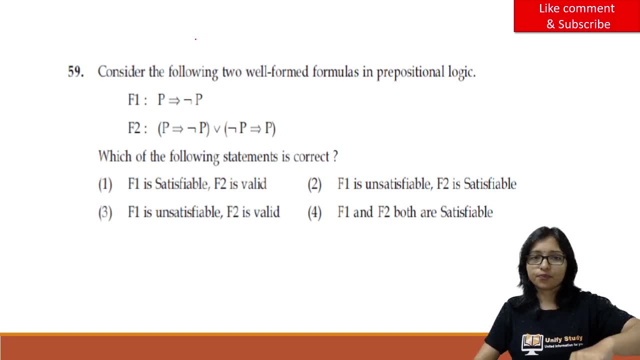 Please let me know in the comment who are here till now. Write down in the comment section: Yes, Now we are going to start the question. Write down that: yes, I learned the concept. Now we are going to start the question, So that I can understand how many students are actually watching this. 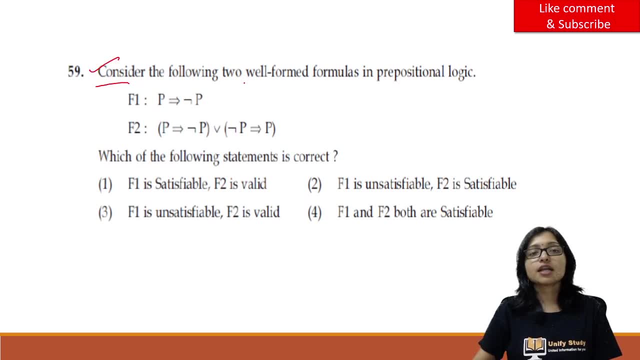 Right. So see, here is the question. Consider: are the following: two well-formed formulas of proportional logic, f1, f2 is given, which one is satisfiable, valid, we have to apply that formula. which one is satisfiable. how to prove it here? just same thing we will apply here. i told that right. p implies q, equals to, not p or q. this is. 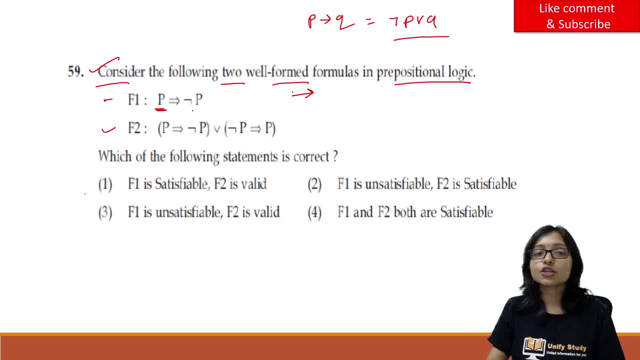 everywhere applied. so here think like that: this is your p, this is your q, so what it is not p, or together q means it is also not p. now it is what actually p bar plus p bar? this is actually p bar plus p bar. so your answer will be: p bar only, right. so when i just coming, only p bar it. 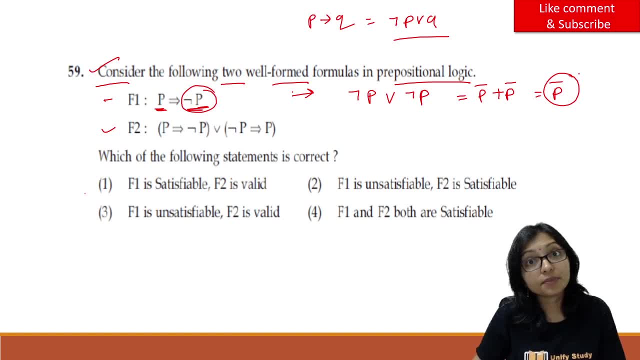 is in a terms of variables. so when i just coming only p bar, it is in a terms of variables. in a terms of variable means, what is it valid? or it is satisfiable? which one? tell me next one how to solve this one. p implies p bar, so it will be not p, or again, not p because it is my p, it is. 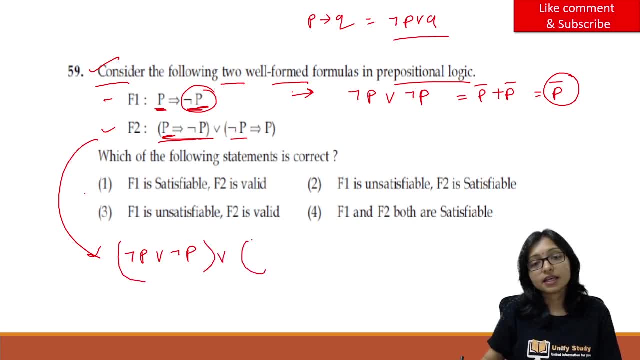 my q here is: or then, not not p or p. now p bar plus p bar. it is actually what? p bar plus p bar, that is actually p bar or means plus. it is double negation: p, p, p, double bar, that is p actually. so it is p plus p means p only. so p, p plus p bar. 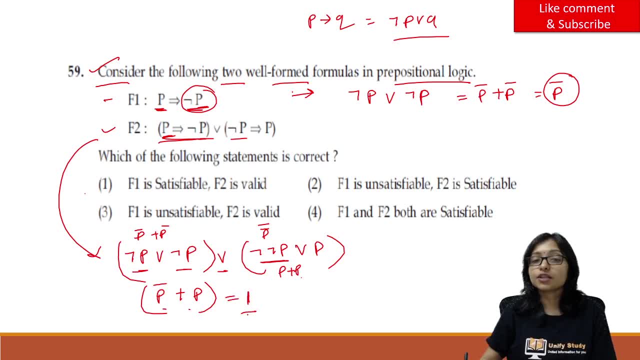 is 1, p plus p bar is 1, so you got here 1 expression giving result 1. that is what? yes, that's why you: it is valid, this one is valid and this one is satisfiable. so answer will be: f1 is satisfiable. 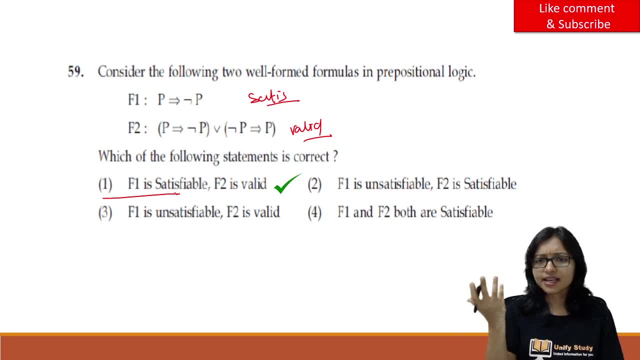 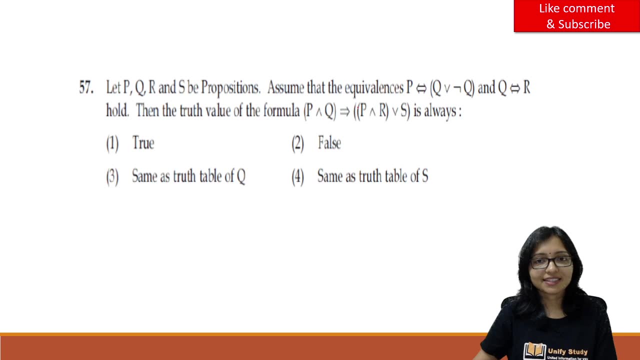 f2 is valid. simple, right, easy. now do the next one. now you can do it right, you can do. yes, you can pause the video and you can try. yes, let's do so. what is given here? p double implication, q or q bar. q or q bar means what? that is, 1, actually. and q double implication- r means in the place of q. 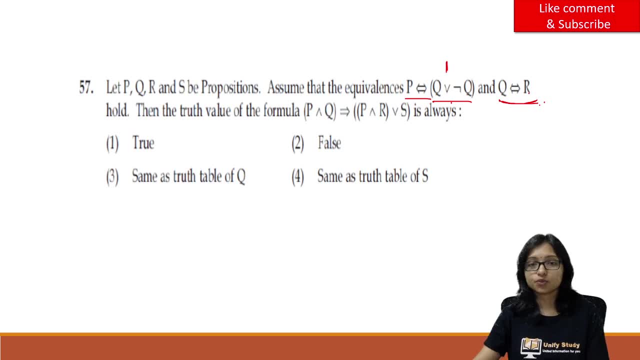 i can write r, in the place of r i can write q. so from here, two things i got: in the place of p i can write 1, actually, and in the place of q, r i can write vice versa. now i need to solve this equation. how to solve? let's try, try it. what i, what i am getting? 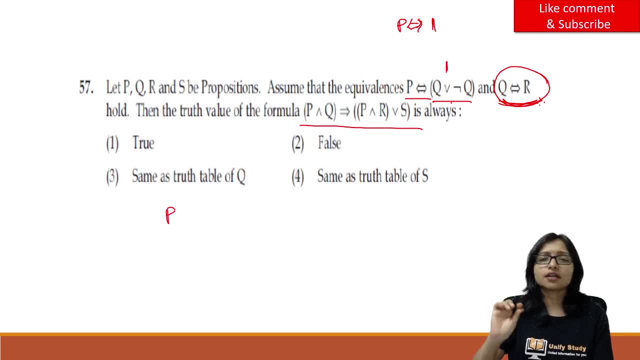 so, first of all, i will write in the form of digital logic, because it is very much good for our eyes, we are very happy, we are feeling very happy because these symbols are really feeling bad. when i am writing in this way, it will be easy for us. so i am writing in this way: p dot q. 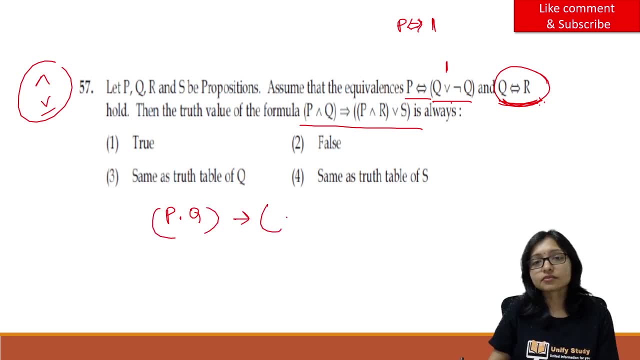 it's done. implication here. the implication was there. now after that we will do here p, dot r plus s. this is here simple, it's done. now see that. can i change anything? is it possible to change anything? in the place of p i can put 1. so in the place of p i am putting 1 here. also in the place of p, i can. 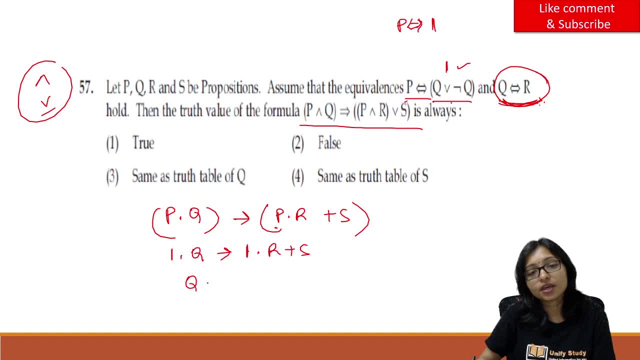 put 1 plus s. so ultimately, what is coming here? q implies r plus s. that is coming right. q implies r plus s. now can i apply this one as p and this one as q? i can do it, this one as p. so it is what? not? q or r plus s? 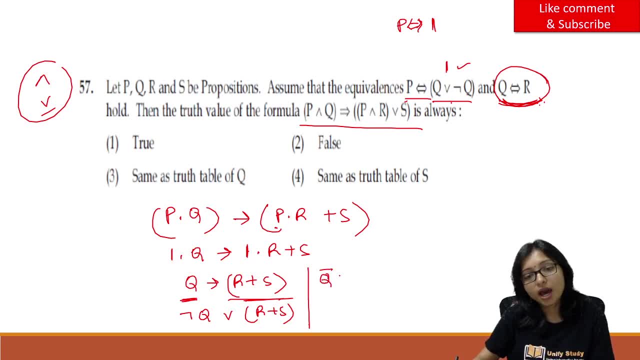 means what it is q bar plus r plus s. right now you can see r double implies q means. in the place of r i can put q. that is q bar plus q S. So Q bar plus Q is what That is: 1. 1 plus S. Q bar plus Q is 1. 1 plus S means 1 plus anything. 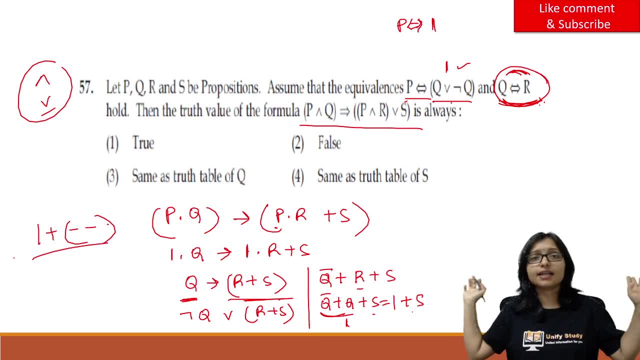 whatever it is. 1 plus infinite number of terms, infinite number of variable, whatever it is, It will be always 1.. Why it is? Because 1 plus 0 is also 1.. 1 plus 1 is also 1.. Is there any other? 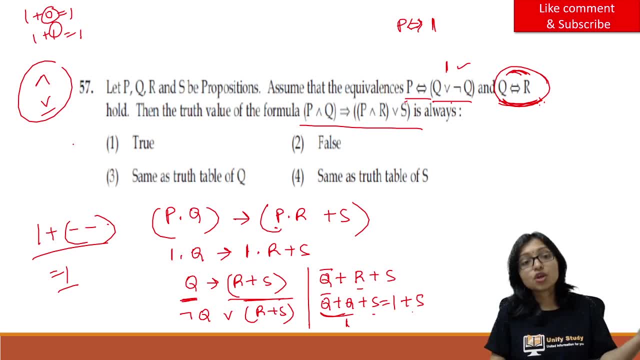 possibility. There is possibility only 0 and 1.. So 1 plus anything is always 1, and that's why, for the time of simplification, try to get 1.. If you are able to get 1, then you can do 1 only. So that's. 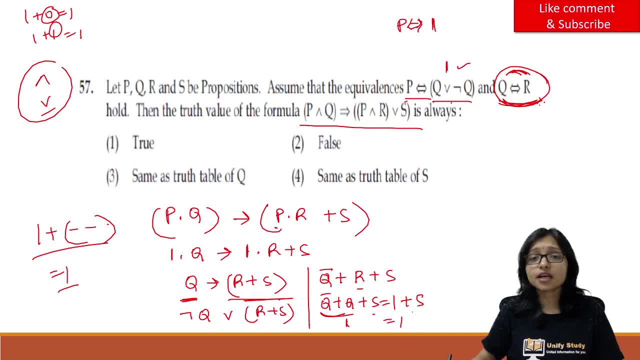 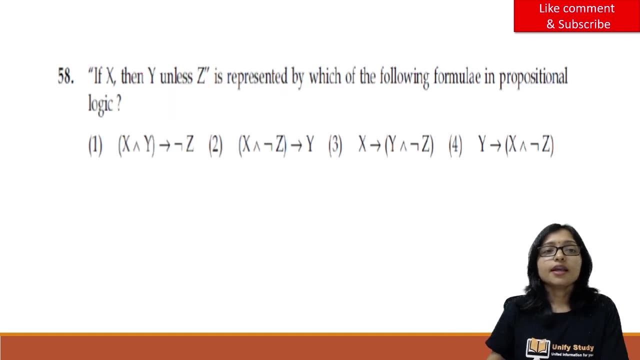 why this will be 1.. And you got your answer. Your expression is giving result. 1 means what it is. It is definitely true. Yes, It's very easy, simple right Now. go to the next question. Here it is: If X, then Y, unless Z. Think it, You can do, Think it. 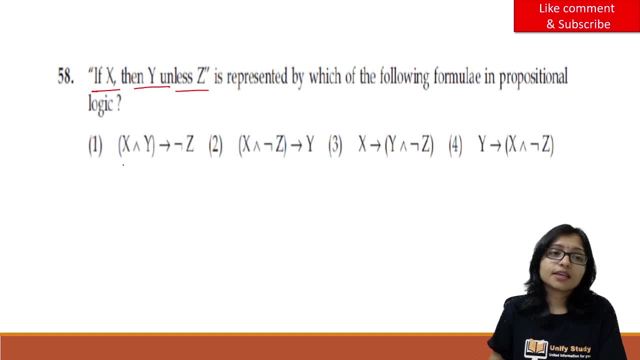 Yes, So you can see here: X and Y implies not Z, X and Z, this one, this one and this one. What is the meaning? Think like that: If X, if it is Monday, then I am, if it is weekdays or if it is. 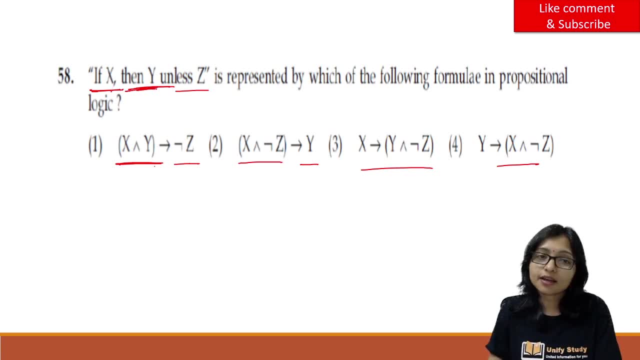 Monday. If it is Monday, then I will take the class unless I am ill. What is the meaning? It is Monday and I am not ill, then I will take the class, Is it or not? It is Monday X and I am not ill. 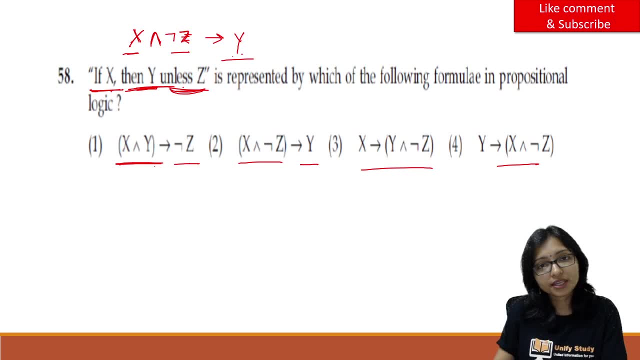 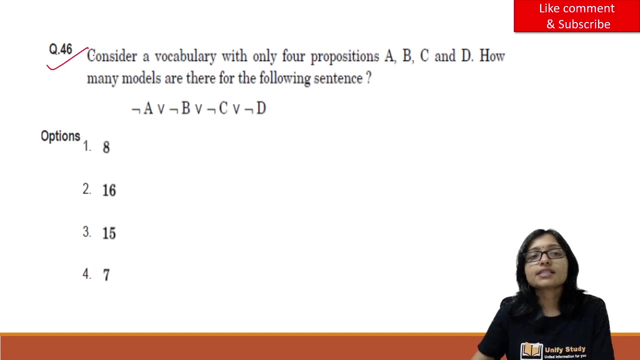 So I will take the class. Yes, It's done here. So this is your answer. Clear Yes. Now go to the next Yes. So this is the question where you have to do the consider the vocabulary Here. this is: what is the model? How many models are there? 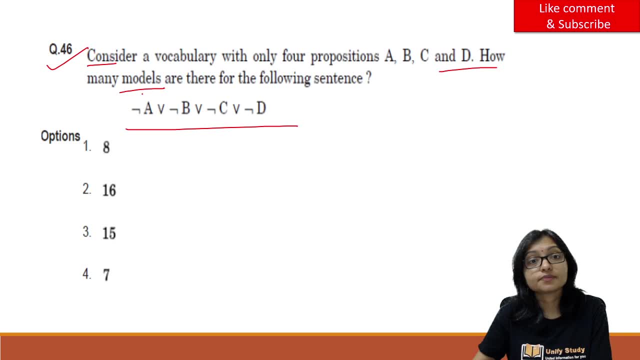 What is model? What is model for you? One girl or 1 boy and 2 boys is 1.. And your type? seconds. We have. What is model? Yes, Model is nothing. Model means, if I am solving this expression, how many variables are there? 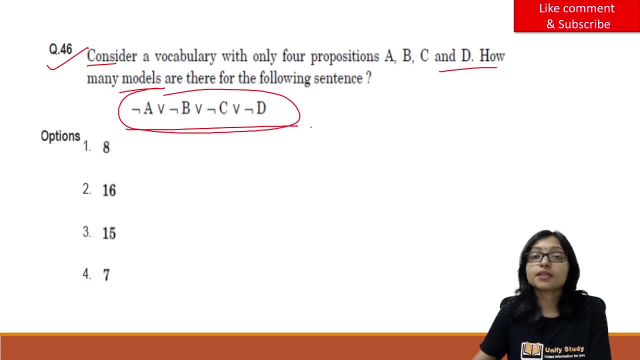 We will make a truth table. Now, in the truth table, how many true are coming That are called model? So, ma'am, there are four variables. I will create the truth table. That will be very lengthy truth table. It is like that. 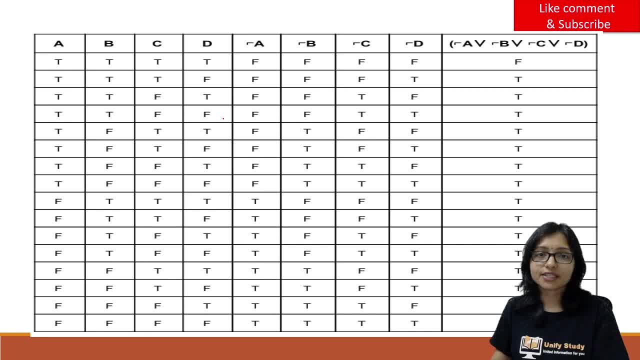 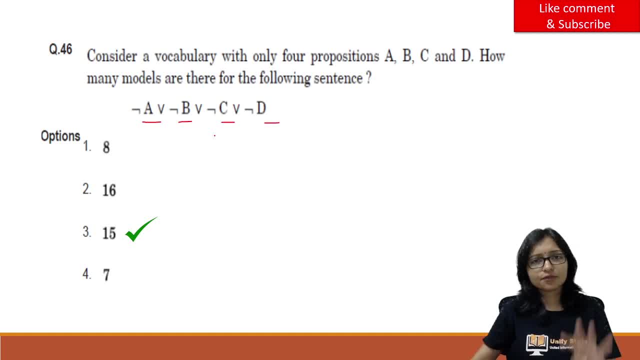 How we can do in exam hall- No need to do it. How to do So? think logically. Think logically Here. how many variables are there? A, B, C, D, Four variables. Using four variables, how many combination we can take? 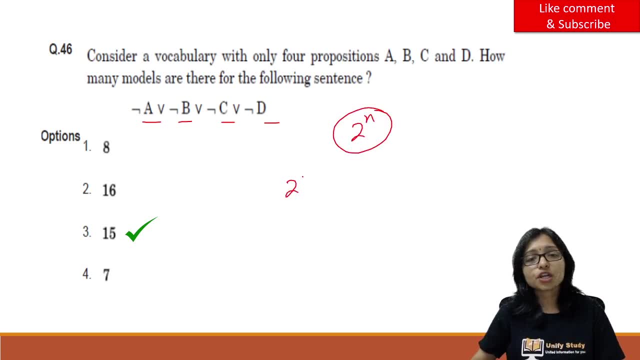 2 to the power n combination, always. So combination will be 2 to the power 4 means 16 combination. Now think that these all are plus right Means or In the or table what is going on? When all are 0, then only I will get 0. 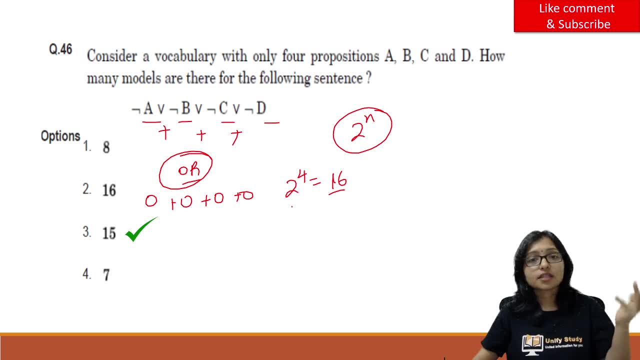 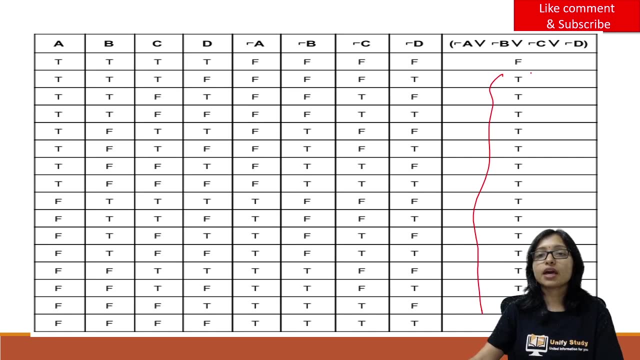 Otherwise, for every combination I will get 1.. That's why I will do 16 minus 1,, 15.. That is going on here, Because all will be true here Only when all are false, then only it will be false. 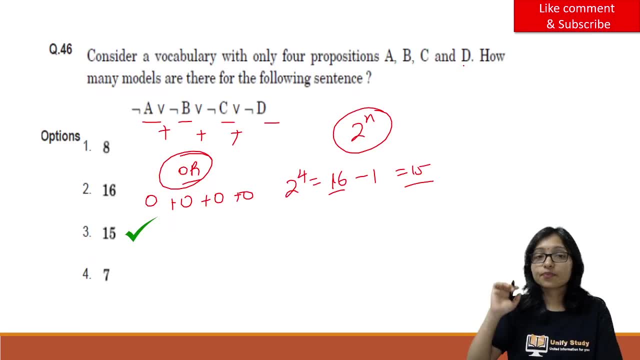 So do it logically, Think it logically. Tell me one thing In this state: if I am doing here, and then what will be the result. Tell me in the comment section. Let me know in the comment section: If in this place I am doing like this, then what will be the result. 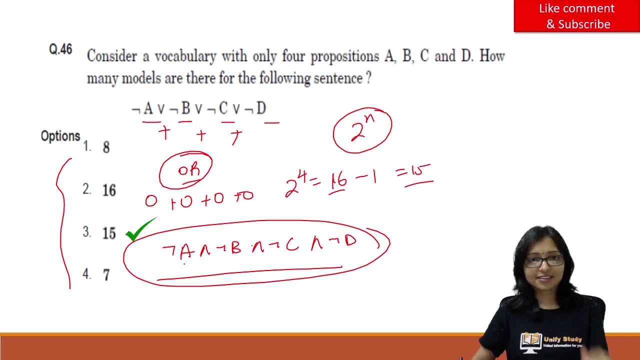 How many models you can create here? What will be the result here? I know I want to know the comment section. What will be the comment section? Okay, See that here the question number. some different question number are showing Because I copy the question from exactly from the question paper. 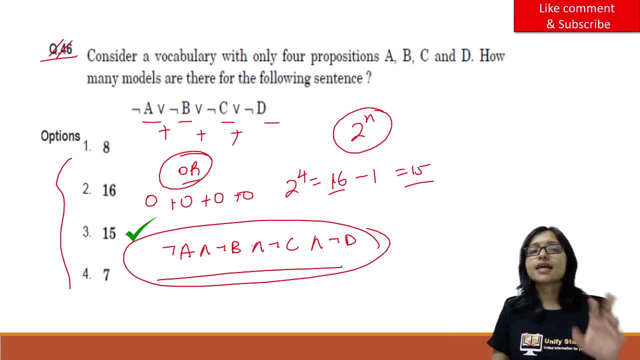 These are the some question of UGC net, some question of gate. That's why this question number is showing. No need to bother, Just write down like that: Be this many models are possible. That is the way I can get the answer. 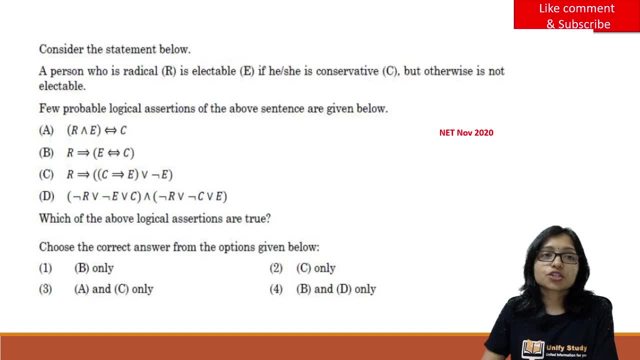 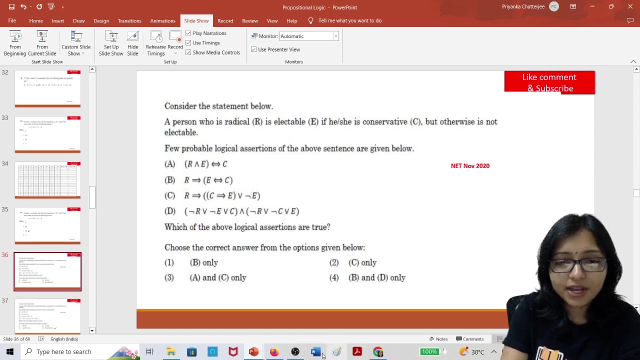 Okay, Now here this question. Do the question, Yes, Do this. and let me check one thing. Technically I am thinking: is it recording going on or not? Let me check once, Do it. Let me check- Sometimes I am doing that mistake also- that, yes, ultimately recording is going on. 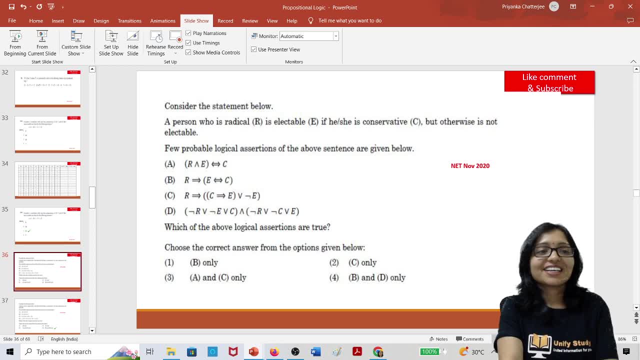 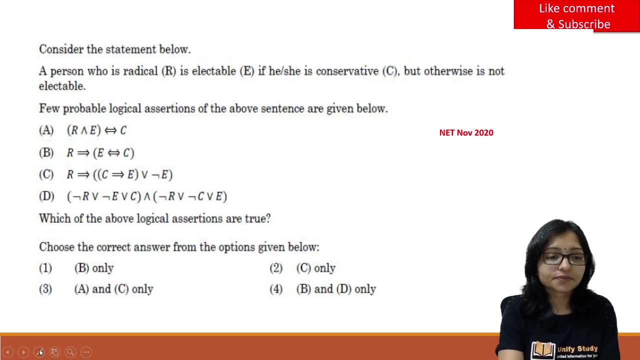 Yes, it is getting my voice. Okay, Good, So I am right. Sometimes I am also feeling crazy. Okay, Do it. So here do this one: How to do A person who is radical and electable if he or she is conservative but otherwise not electable. 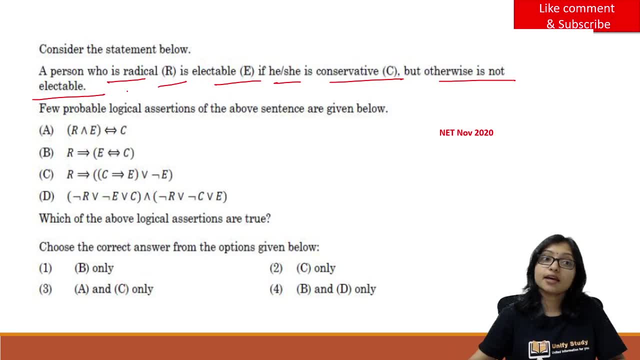 What is there in if Think, Do it, Do it, Think it. Yes, The answer will be this one and this one, Ma'am. why this is the answer? Because see that what is, if a person who is radical a person is radical, that implies he. 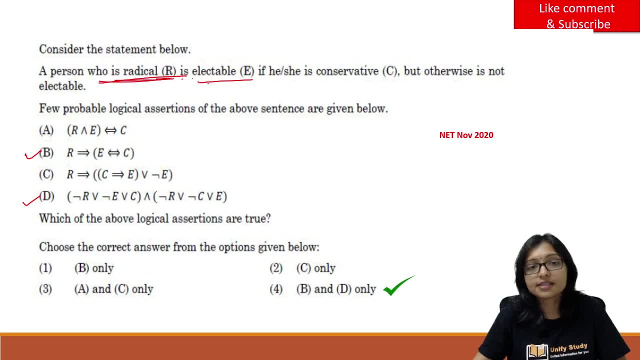 is electable. So this is my P, This is my Q. So implies who is, implies the person. if the person is radical, that's why the person is radical. implies electable, Implies electable, implies electable. There is another condition also: that if he is conservative, that's why, if he is conservative, 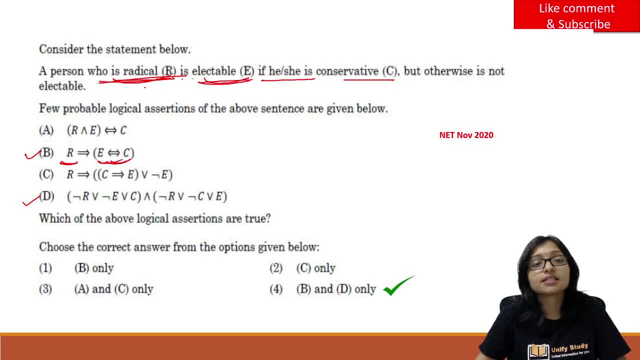 it is actually if, and only if, the person is electable, then he is conservative, and conservative means electable means it is radical. So that's why this is correct. Why this is not correct, ma'am: It is telling you the person is radical and electable. 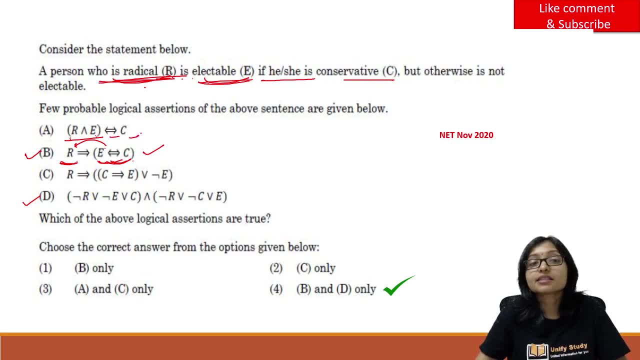 That double implication. conservative means. here it will be. a conservative person is always electable and radical It may not. I told you always that when I am telling P implies Q means, it does not mean Q implies P. A person is radical, is electable, if he is conservative. 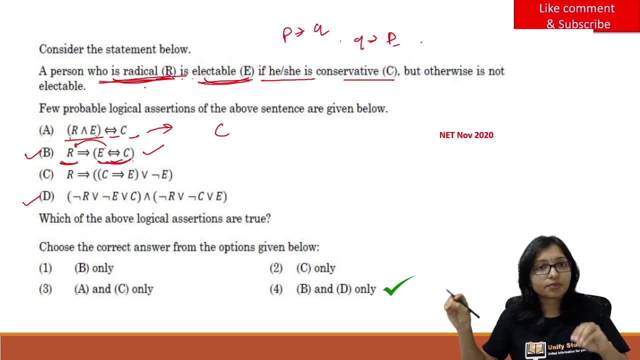 So there is a person who is conservative, radical, that person is electable. That does not mean that every conservative person is electable and radical. That's why this is wrong. Now, ma'am, how to get D? D is actually the implication going on here. 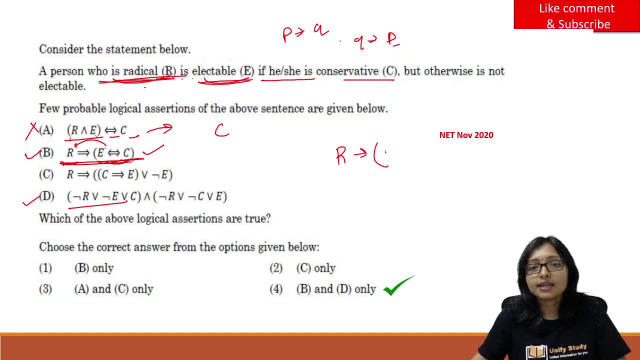 What is the implication going on? R implies E, double implies C. It was there Right. So R implies D means this is your P, this is your Q, Inside the Q, what it is. double implication means E implies C And C implies E. 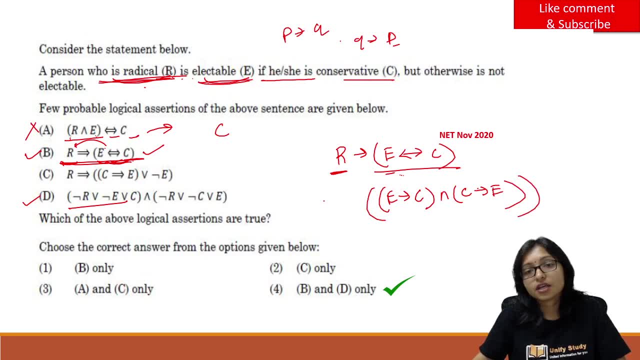 That is the meaning of double implication. And outside that is R, So it is your P, this is your. Q means not R or this part. Again, this will be not R or this part, So it is actually the expanded format of B. That's why answer will be B and D. 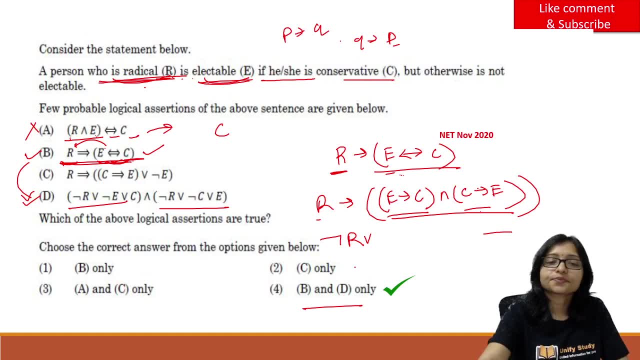 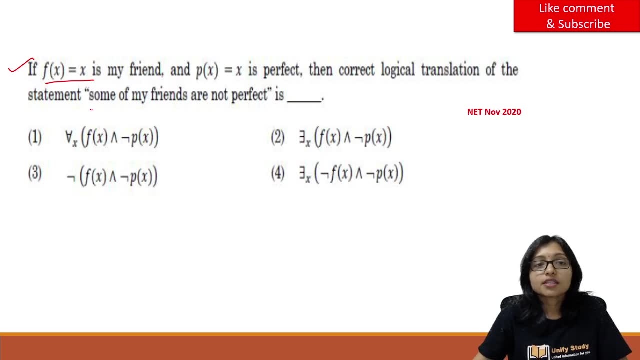 Clear. I hope this is clear. Now see that here it is another question that F equals to X. Some of my friend are not perfect. Some of my friend are not perfect. What to do? These are actually the predicate logic question. So I am telling you predicate logic. 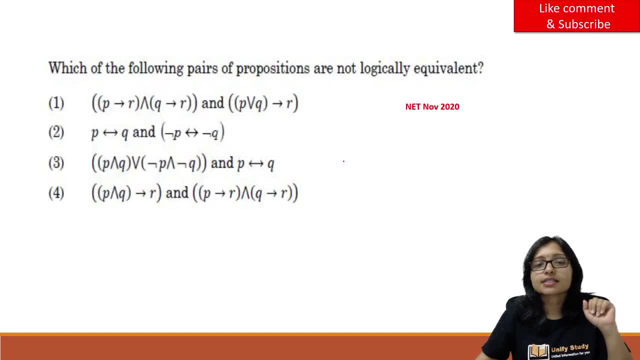 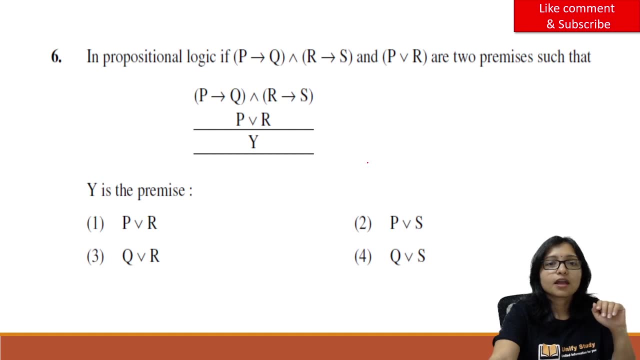 After that, we will come to this And these are some home talks for you. You can do it and this is the answer now. Now you can do this question. So this one is a Syllolism. Do this one. What is a Syllolism? 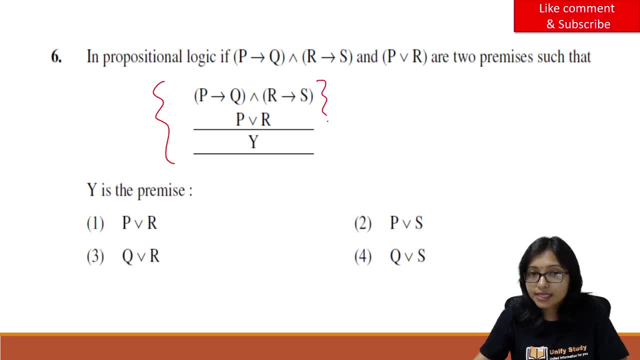 How to prove it. Actually, these are given to you. When these are given, then what will be the value of Y? That is, you have to know What is the value of Y. P implies Q and R implies S, And it is given. 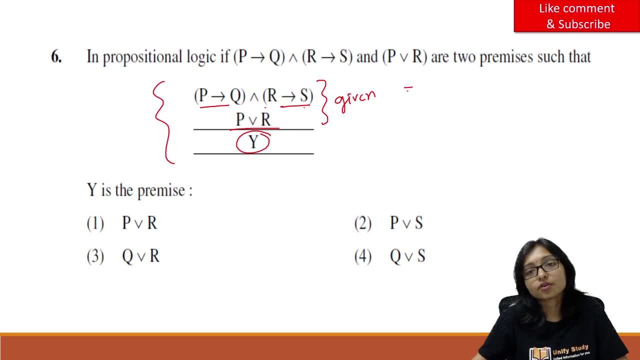 And it is given that P or R, What is this actually? Not P or Q And not R or S, is true given to you? And another one is given that P or R equals to 1.. So see that This total is 1 means this part also have to be 1.. 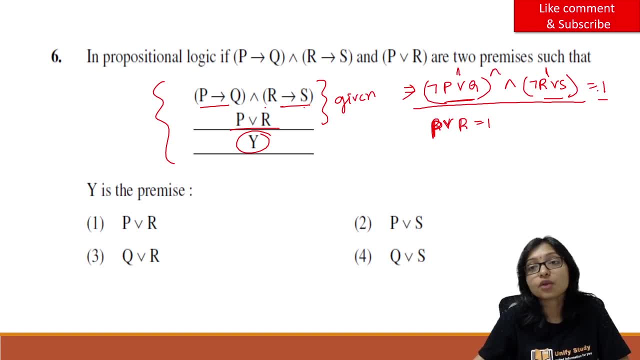 This part also have to be 1.. Because and means when both are 1, then only it is 1.. Now, when P is 1, then P bar will be 0. Then Q have to be 1.. When R is 1, then R bar have to be 0. 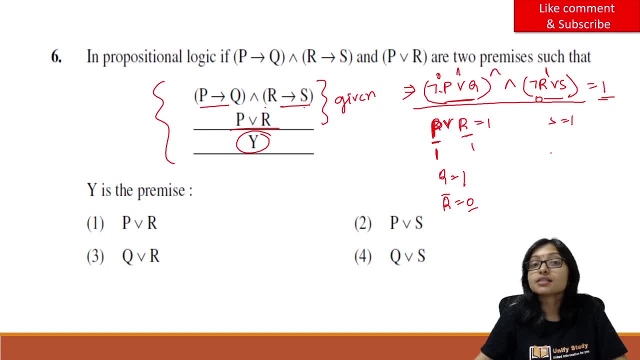 Then S have to be 1.. So what is the meaning? Either R or S, Either Q or S are not Q, Either Q or S have to be 1.. Otherwise I cannot get it 1 right. When this part is 0, it have to be 1.. 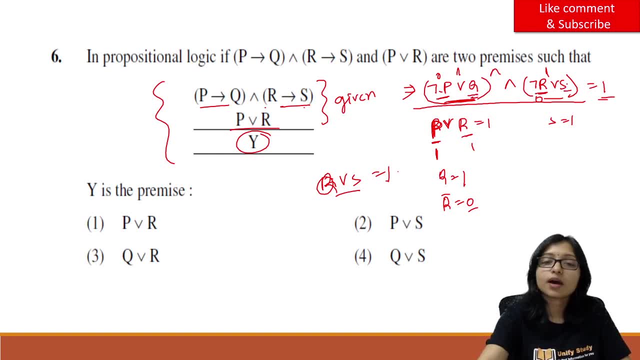 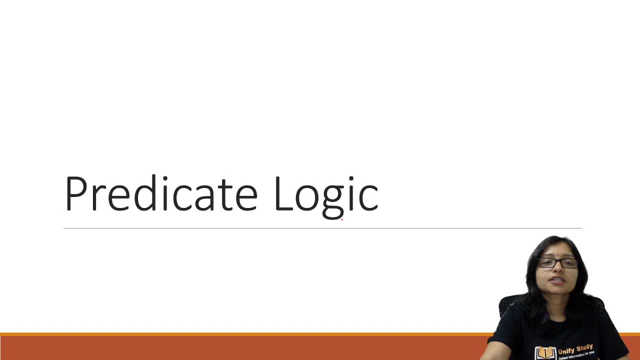 When this part is 0, it have to be 1.. So that's why either Q or S have to be 1.. Yes, Got it. Now we will do the predicate logic. In predicate logic there is two things. One is there exist. 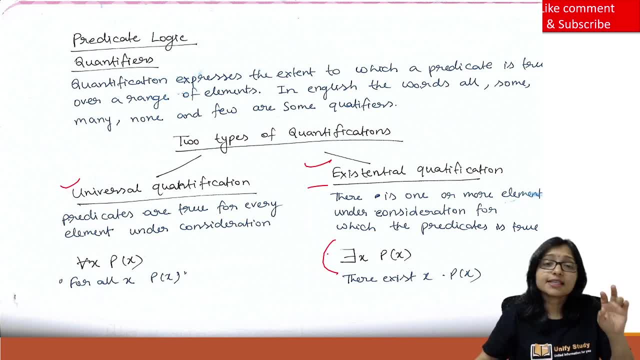 Another is for all. There exist means at least one element is true, Some of them, Some of them, or one element is true For all means everyone is true. All the student of this class who are watching. They are the computer science student. 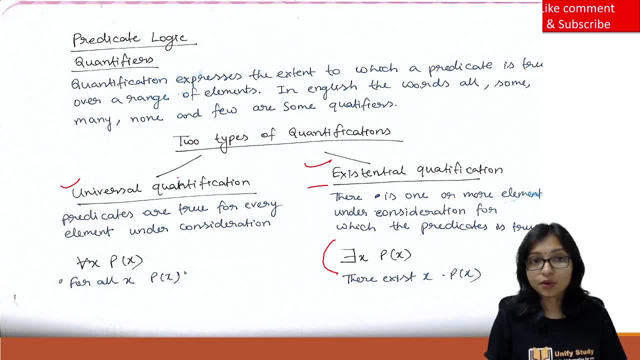 Right Or there the mathematics students can be also, Because in discrete mathematics is there Those who are. They are the discrete mathematics students. There exist means There exist some students, Some are male, Some are female. There exist, That is, there exist. 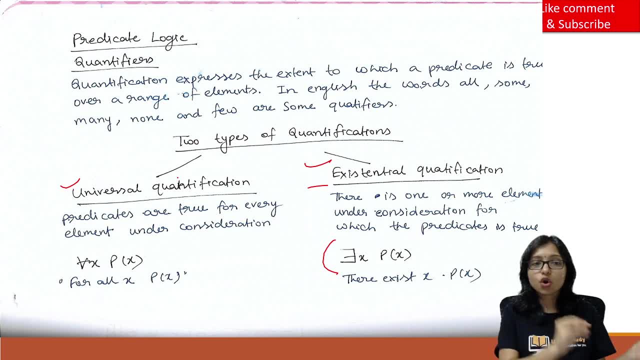 Some of them, Some of them, And it is all of them. So all means for all We are writing in this way, There exist means there exist in this way. Now, whenever I am writing for all there exist, Then we are comparing with a variable. 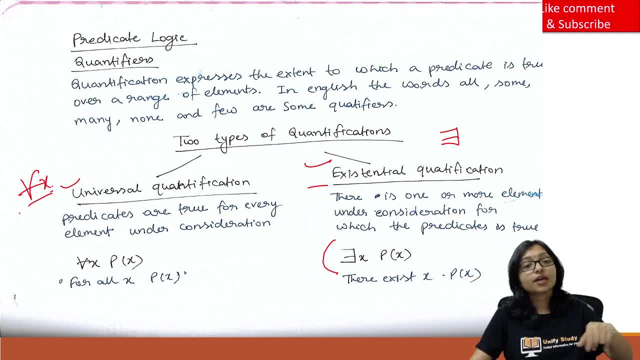 X is a variable. That variable will be compared with a domain. That domain is the class. So in this class all students are discrete mathematics students. In this class- That is PX- Some of the students are female. That is the comparison. 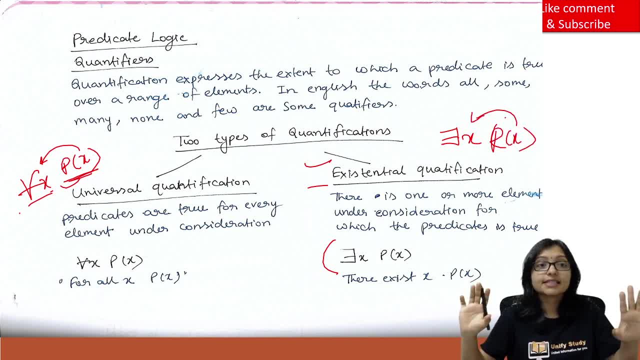 Always we are comparing with a domain, In a specific domain we are comparing. So now, here there are something, What we can do For all means. lots of thing are possible. All of them For each Given any, For arbitrary, For each. 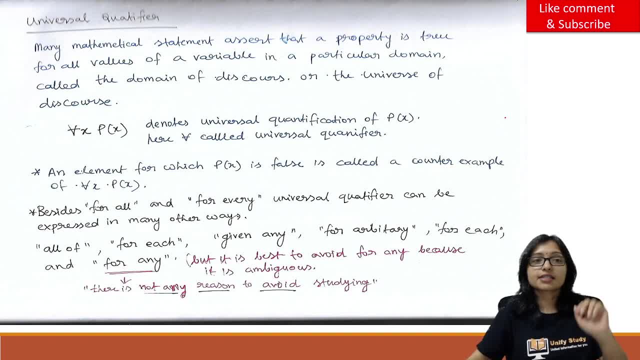 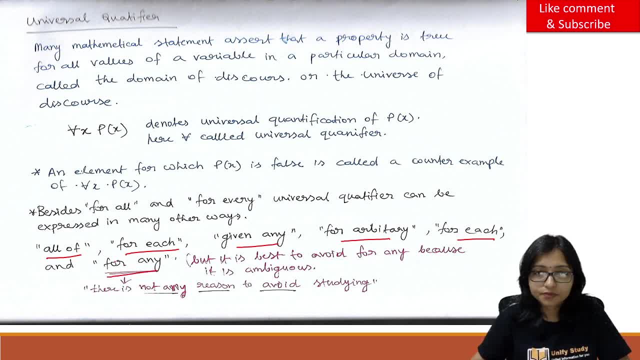 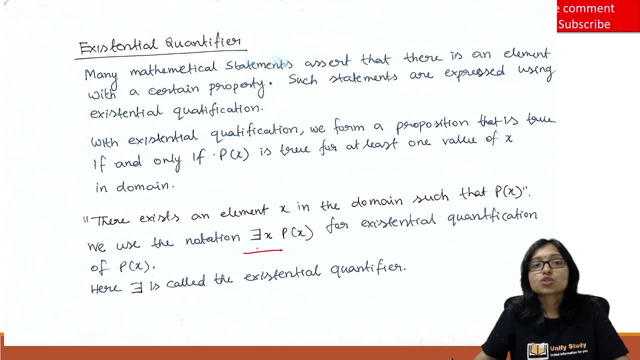 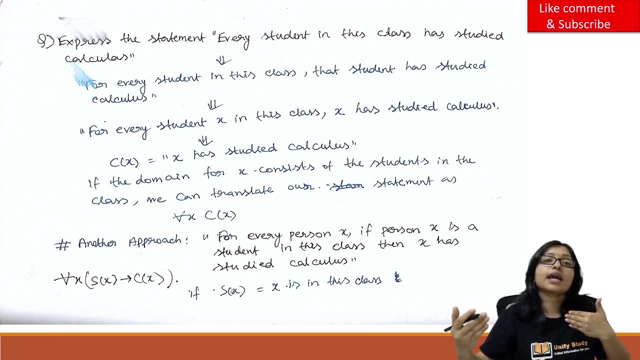 These all the meaning are actually for all and we can write like this way. Another one is existential, that is, their exist. So for their exist means at least any one of them is true. So many different way we can express that. every student in the class has studied calculus. 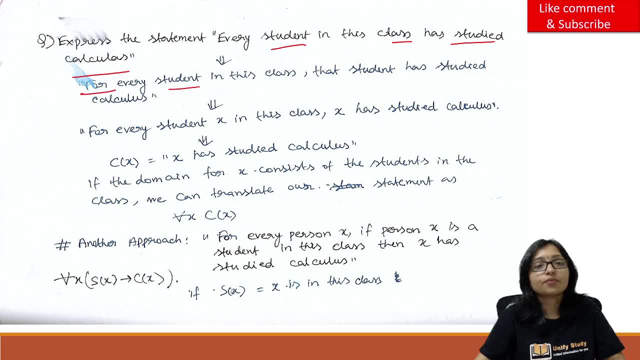 The same thing we can express like that: for every student in the class that studied calculus. for every student x in the class x has studied calculus. so if i am telling cx is the predicate that x has studied calculus, then how to represent for all x, cx. this same thing we can represent in: 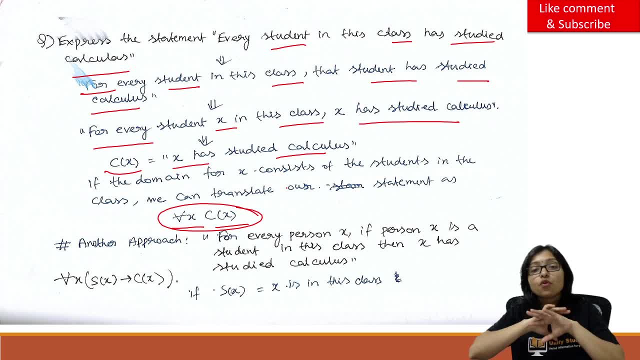 another way if we are trying to do for the total world, for every person, x means any person in the world x. if the person x is the student in this class, then they studied calculus, then they studied discrete math. if i am telling this same thing, we can represent like this: now the for all x. 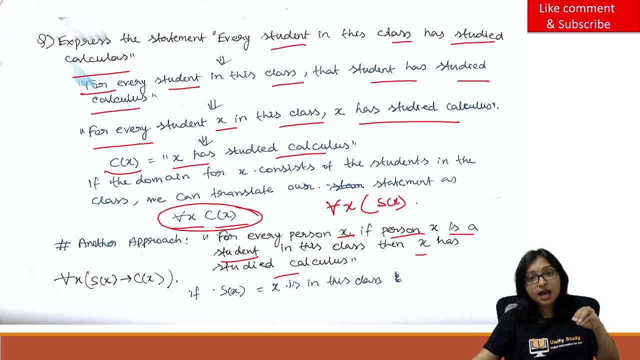 if the student, if it is the student of this class, then they studied this. calculus means, i can say discrete math also got it. so it is a trick. remember you. Whenever we are using for all, most of the time for all will be we can represent in the there exist format. means this implication format. 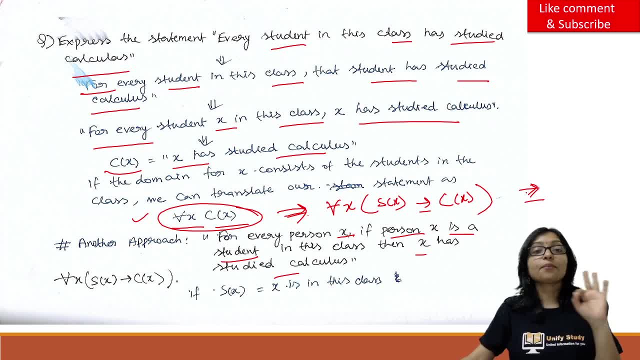 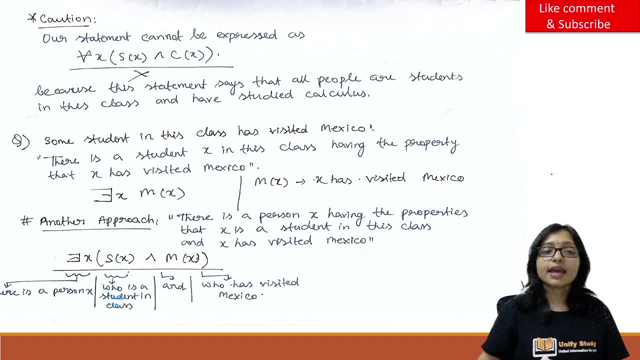 Here only. this is the trick. in this trick, you can apply everywhere to solve the question. with the for all, we can use the implication And here, whenever we are doing, there exist, but here, with the for all, we cannot use the and we cannot use the and with the for all, because this meaning is different. 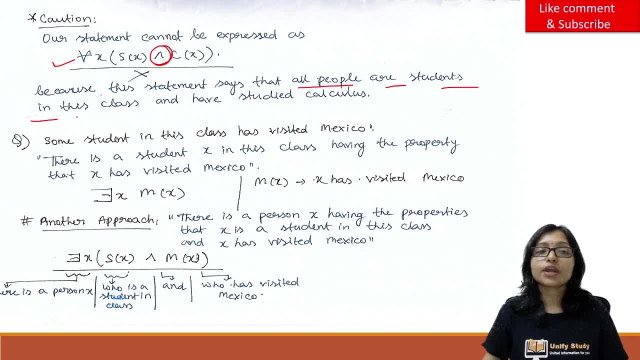 It will. this statement will say: all the people are student and the class studied calculus. all the people throughout the world. I am telling they are my student. no right. That's why, with the for all, we cannot use and But In there exist. whenever I am writing, there exist. some of the student in the class visit Mexico. some of the student in this class are female. 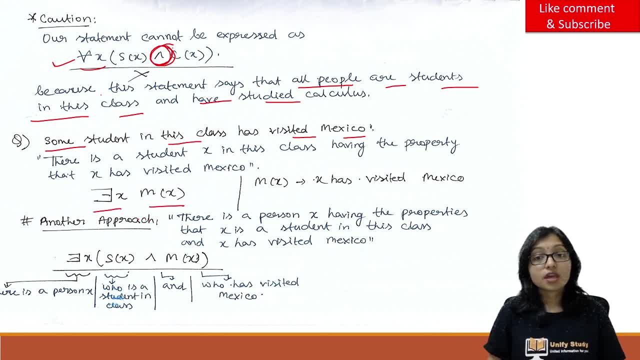 Then we can say there exist MX. So MX means visited Mexico. This one we can apply and there exist some. there exist X, They are the student and they visited Mexico. So with the there exist, we can apply. and This is The trick. if you are able to remember, then so many predicate logic question will be easy, because here only students are getting confused where to use and where to use implication. 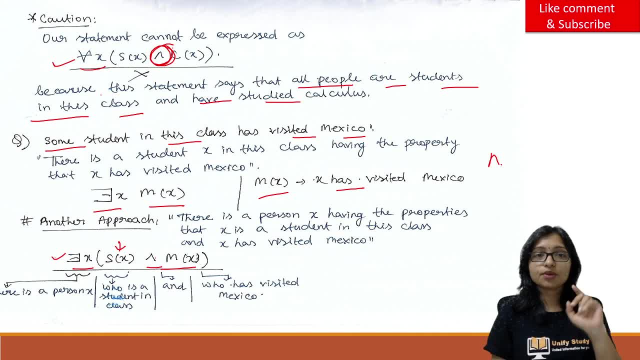 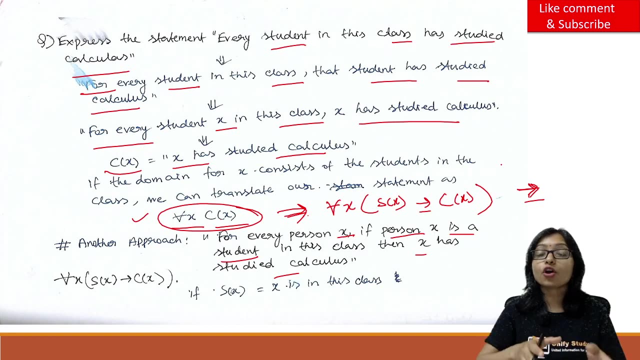 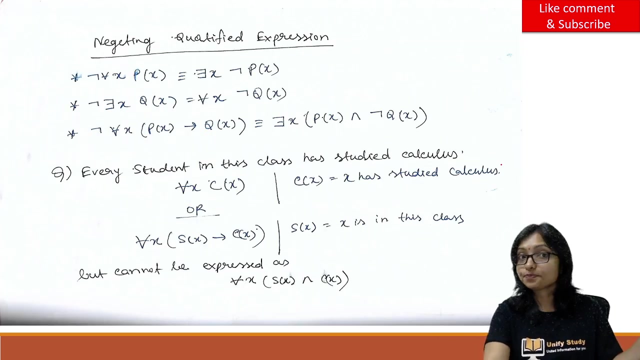 Where there will be, if then condition, then we will apply implication, and where there are, we are trying to combine two: statement, then it is, and, and most of the time, with the there exist and will be applied, and with the For all implication will be applied. this is the trick to solve this type of all question. whatever I shown, 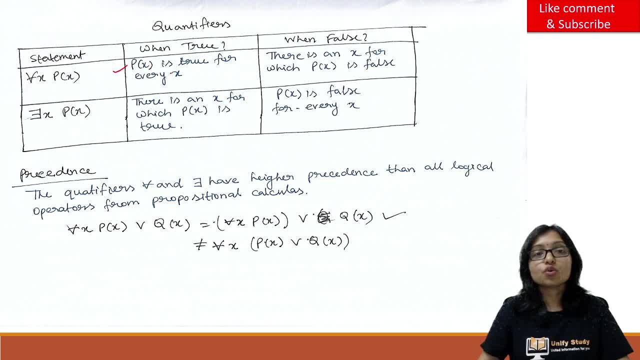 Now you can see here. that is that this is the way it is true. when all are true, then it will be true. when it is false, when he is anyone is false, then it will be false. right there exist. when it is true, if anyone is true, then it will be true. if everyone is false, then it will be false. 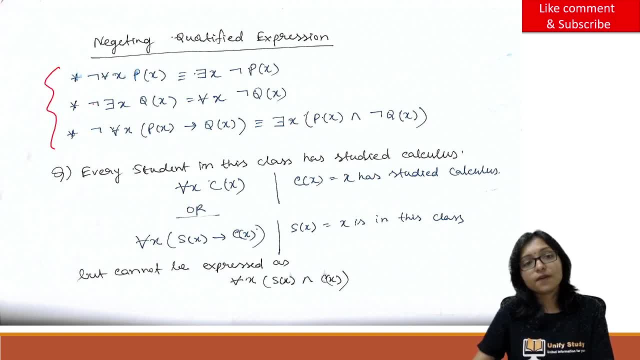 Now see, These are the three very important rule. if I am applying negation with for all PX, then this will be changed to there exist and this will be changed to not be. If I am applying negation with there exist, this will be changed to for all and this will be changed to negation. 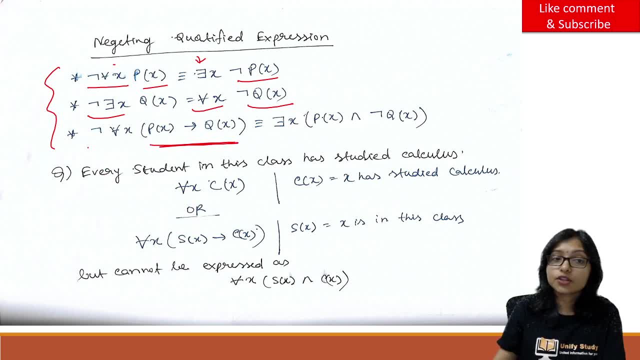 And this P implies Q, actually not for all- will be changed to. there exist and this one is changing to, and why? It is because just expand it. it is not PX or Q, X. right now I am Multiplying, not so negation, negation, PX will be PX only, and or negation will be changed to and when I am negating or means negation is doing with or then it is changing to and and this will be. 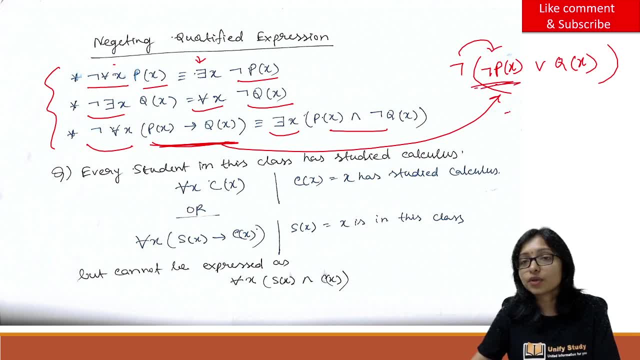 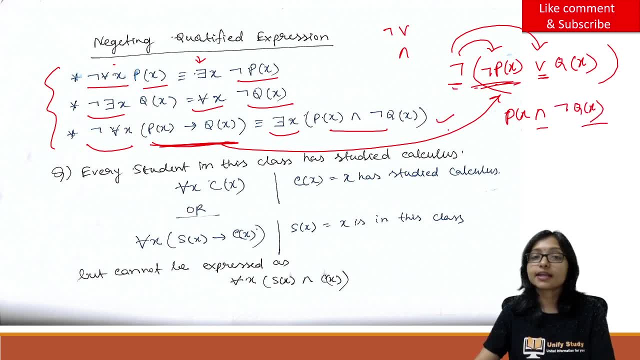 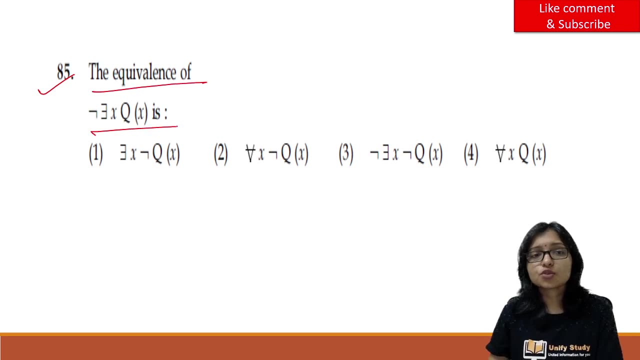 Px, or this will be not qx, And that is why will get this one. these three are very important for doing the predicate logic right. So let's do now The equivalence of this one. just now I told, yes, you all are correct. Just now we did it. it will be for all and this domain will be multiplied with this one. 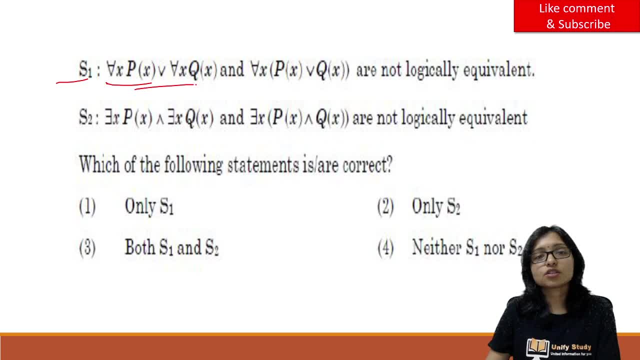 Now see here, Here for all x, this one and this one not logically true. this one, this one, are not logically true. which one is correct? yes, both are correct, because why i am comparing with this domain? these are the domain of male, so all x are male here. or these are all x are female here. 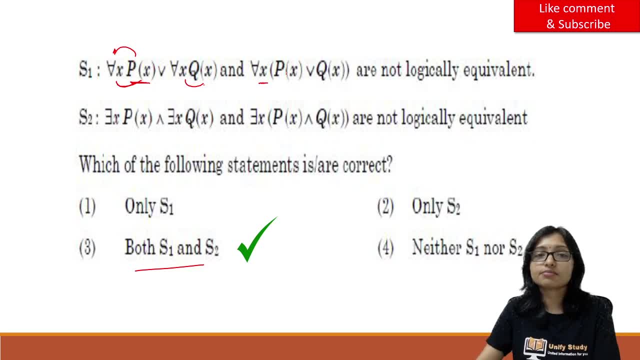 i cannot say there is a specific person. i am telling and it is male or female. this is not true. means this domain? it is according to this domain. this is according to this domain. i cannot say. maybe these are the computer science student, these are the x are the computer science student. 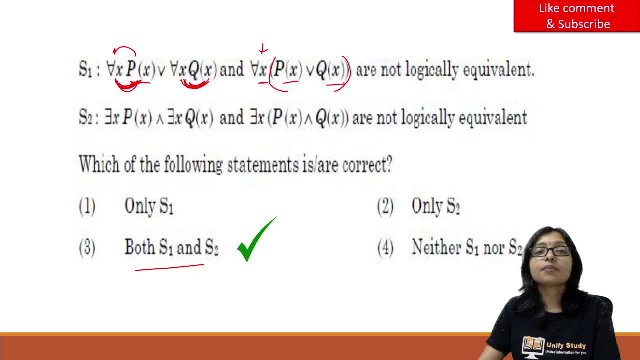 these x are the economic student. now i am taking a person and i am telling: no, it's not equivalent. here also there exist x. there exist. so i am comparing with this px here it is comparing with this qx. i cannot say and means both is true? no, these are also. 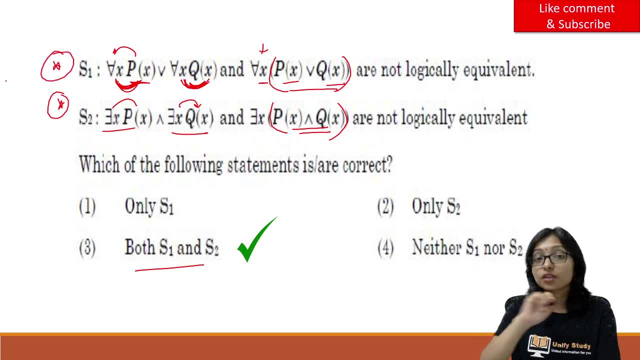 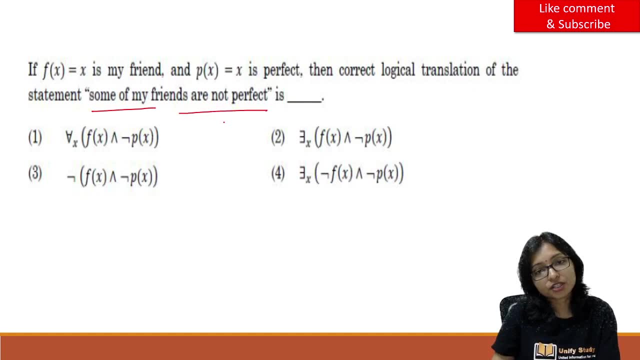 actually very important to rule of predicate logic. note it down. now we can do the question. some of my friend are not perfect. some of my friend are not perfect. how to do? yes, there exist x, they are my friend, friend, they are my friend and not perfect. ma'am, why? this is not the answer. it is telling you for. 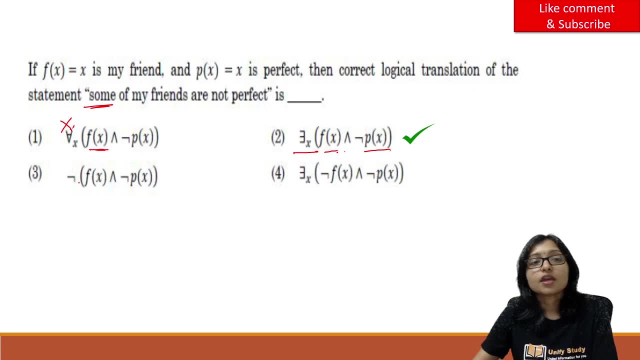 all, it is not some. so it cannot be the answer. here i am telling not. here is no x. x should be compared with the domain and this predicate is totally wrong. here i am telling there exists. they are not my friend. the person have to be my friend. they are not my friend and not perfect. 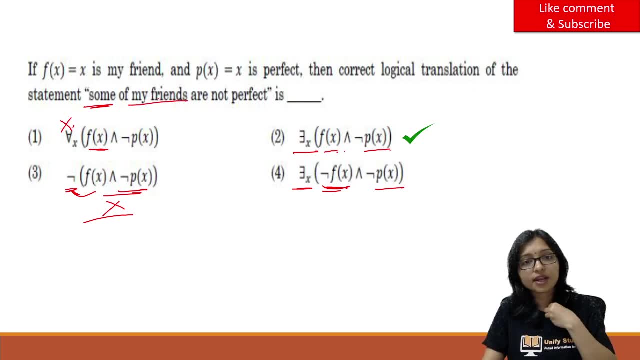 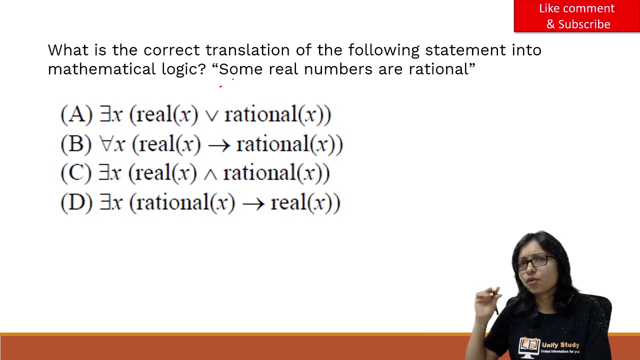 this is not implying this. the person is my friend, then only i can say: it's not perfect, it is not my friend. how it is possible? that's why this is wrong. got it now. do this. who are watching till now? give me, give me comment section. yes, this time i am here, i am present, present, ma'am, because from a long time i am. 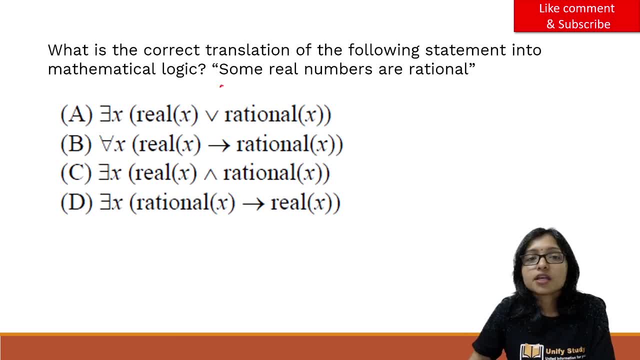 talking. you are listening or not. some real number are rational. how to do? some real number are rational. some real number, yes, some means there exist. it cannot be for all. now should i apply implication or- and i told that with that they are exist, we should apply and this trick will be applied. you. 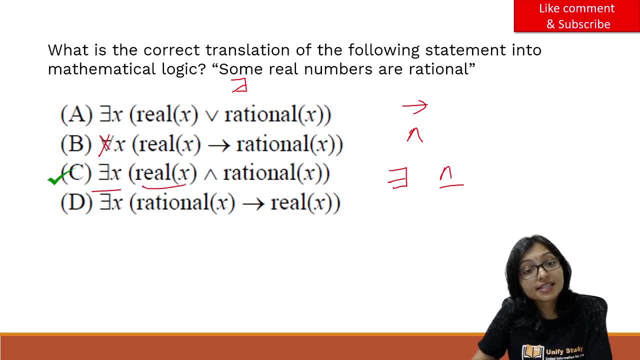 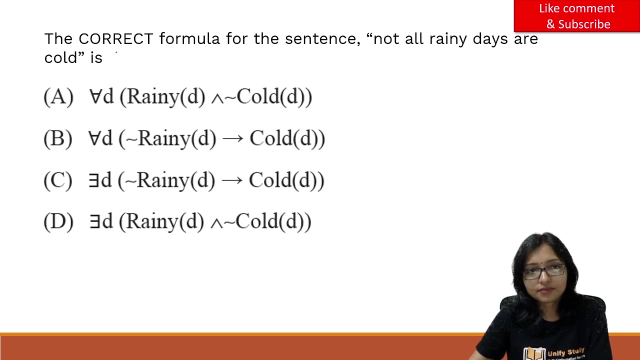 can see. yes, there exist x. this is the real x and rational x. real x and rational x. it's done right with the trick. it's very easy. otherwise you will think that why it is not? because there is no. if then and there exists, we should not use this. you learn it now. see correct formula for. 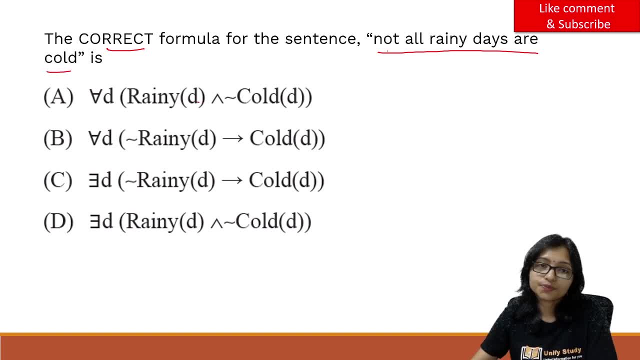 not all rainy days are cold. how to do? not all rainy days are cold? yes, not all. it's not all. not all means negation for all that will be changed to. there exist not all. some of the days are cold. some of the days are not cold, maybe, so not all means that will be. 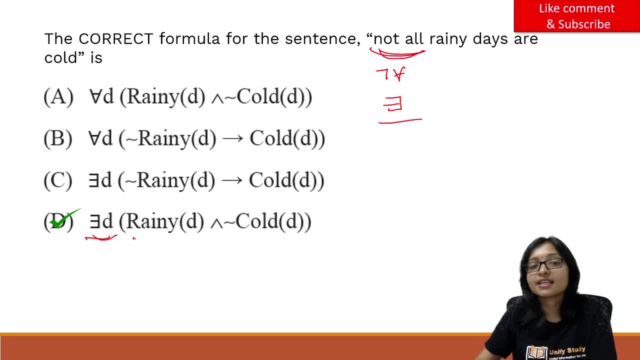 there exist. and whenever i am telling there exists, then it is in any day and it's not cold. you are telling here: it's not in any day, it is not correct. here i am telling for all for all. it's not correct, it is the correct one. 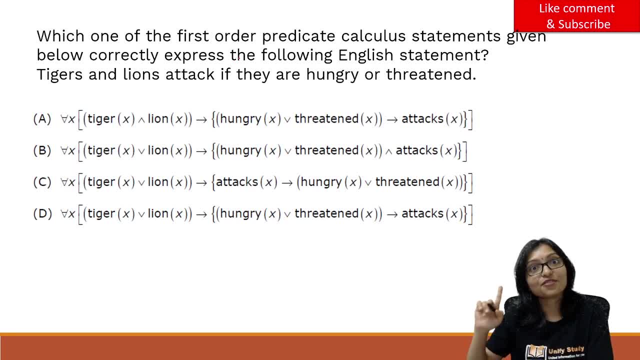 now the next one. do this very carefully, understand it. tiger and lion attack if they are hungry or threatened. tiger and lion attack if they are hungry or threatened. how to do here? you all are doing a common mistake by looking this and you are searching the and symbol and you were doing here mistake. yes, that is. this is wrong. 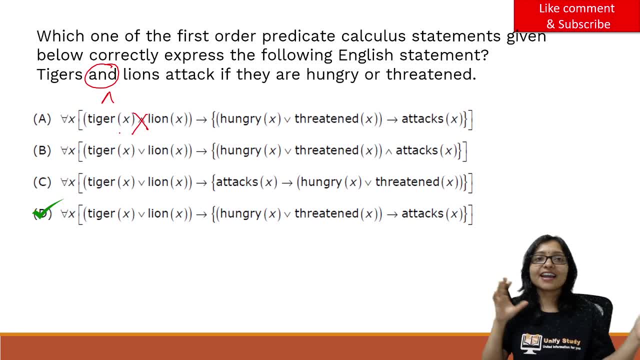 why, ma'am? because see that tiger and lion means either time tiger or lion, they will attack. it's not like that. a tiger is hungry. it will call the lion: lion, please come, we should go, for we should attack. it's not like that. what is the inner meaning? either, it is tiger. 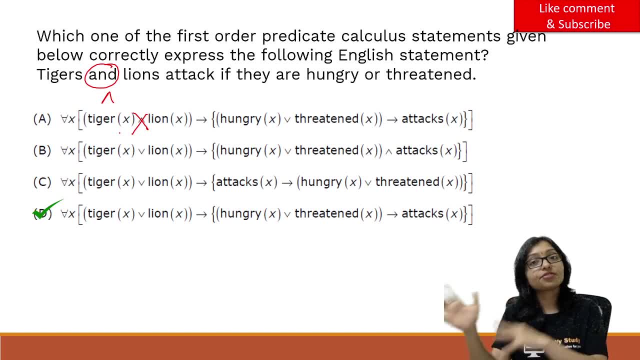 tiger and lion, or it is lion. they will attack if they are hungry or threatened. that is the meaning. understand the meaning of the student or meaning of the question. it's not and it is, or actually so. either it is tiger or it is lion. if it is, then they are hungry or threatened, then they will attack. 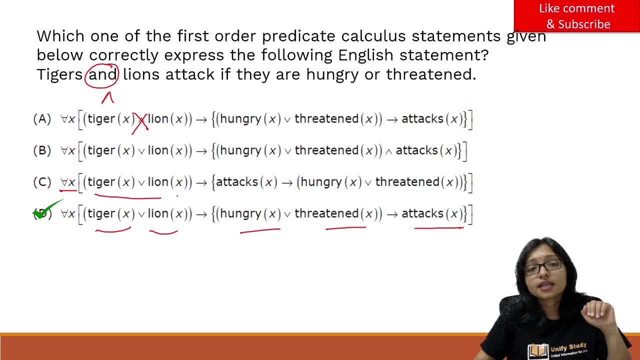 right why this is not because for all there exists attack, then it is opposite: p implies q does not mean q implies p because they attack. it does not mean they are hungry or threatened. maybe it is for any other reason. maybe you are attacking the child of that, or maybe. 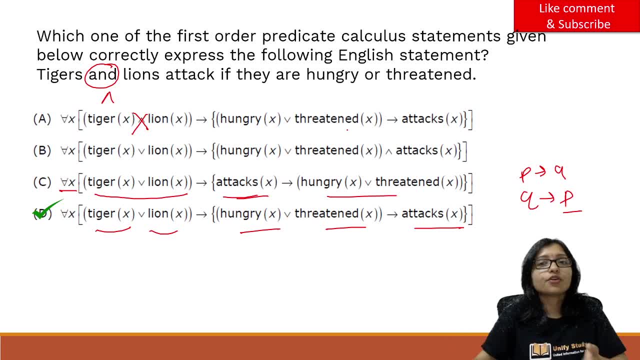 any other reason can be also there. so we cannot say: p implies q means, q implies that is hungry or threatened, then only, it is your p part, it is your q part. this one is that's why not true, and these are two definitely not true. it is not for all, or i am telling here all. 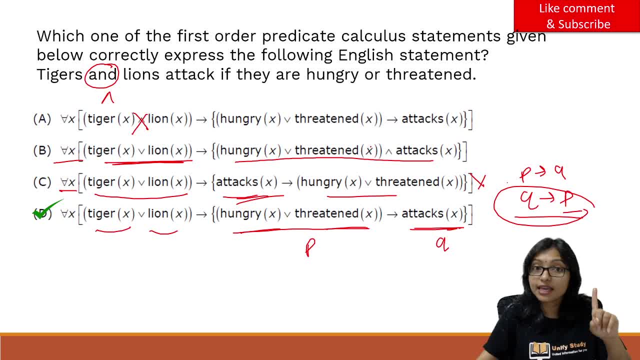 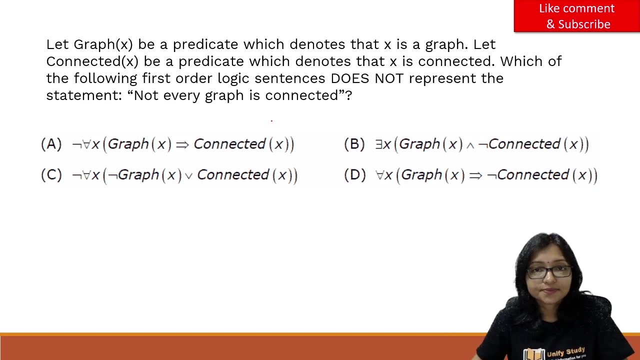 are or no it's have. if, then condition is there. if they are hungry and threatened, then they will attack. so with the or we cannot cut it. this is a very interesting question. i hope you can understand now do this one? yes, not every graph is connected. read the question very carefully. 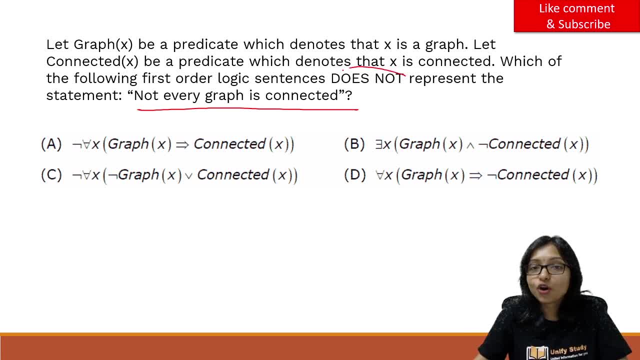 yes, there was a, not very carefully checked that it does not represent this one. which one does not represent this one? so not every graph means what. that is definitely not for all. definitely it is not for all, so not for all. ex. if it is a graph connected, it is true, not all graph. 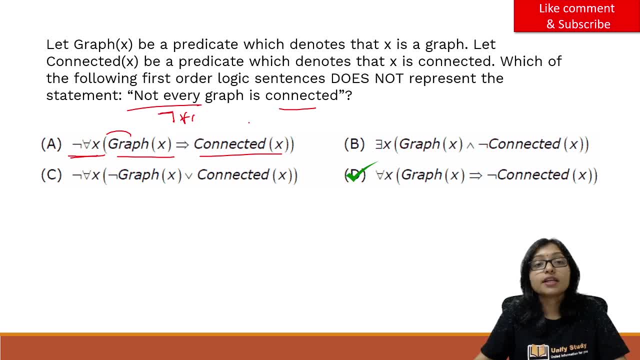 connected, not for all, is changing to their exists. so that's why it is their exists. so that's why it is their exists. is there exist? if i am doing just just solving its x, p implies q, then it will be this one right and not for all x. it's not a graph or not connected. that is also from here. i can implies. 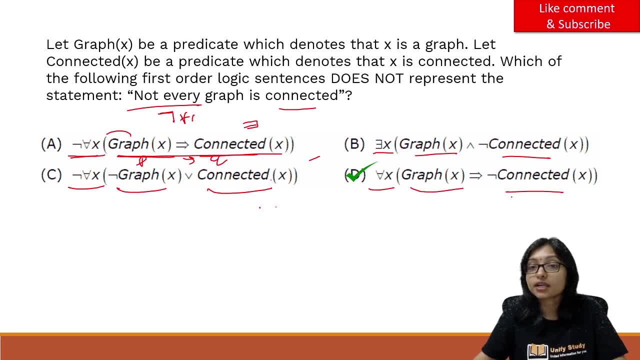 but here for all graph not connected. here i am telling all graph are not connected. no, not every graph means some of the graph can be connected. so i cannot say that all the graph are not connected. that's why this was wrong. it is asking you does not represent means out of them. 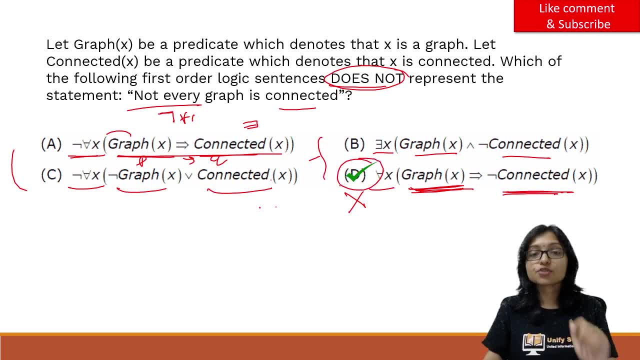 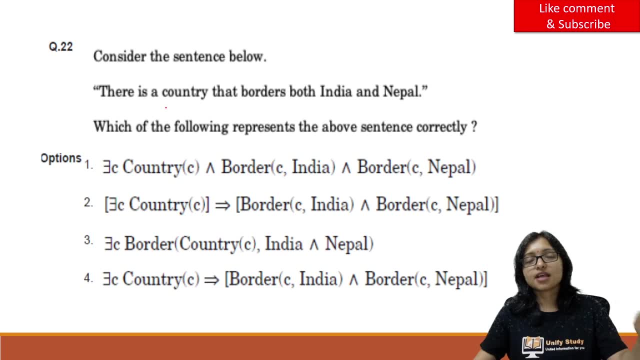 which one is wrong. this one is wrong. that's why answer will be this one. yes, now this is a very popular question. two times it sucks in you just in it. you can see here there is the. you can see here there is the. there is a country that border of nepal, india and nepal. what will be the answer? 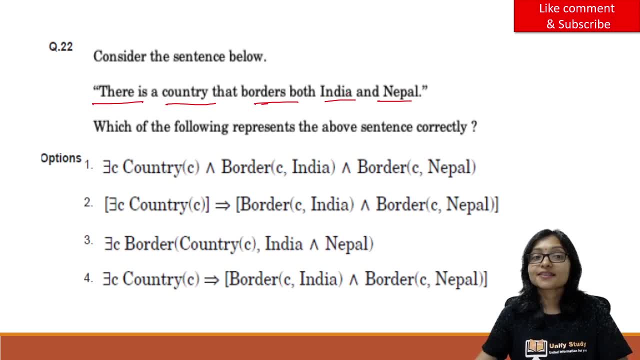 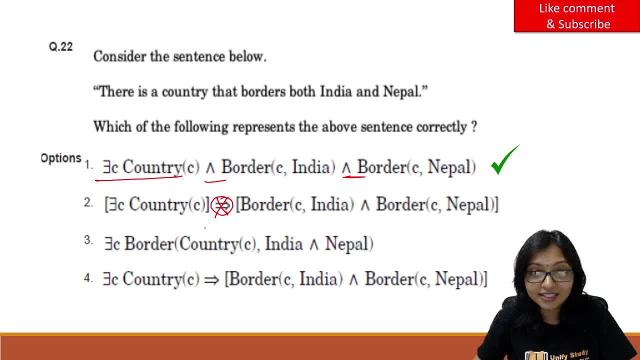 is not. it's not equals. there is a country and it is a specific country that country is the border of. is not, it's not equals. there is a country and it is a specific country that country is the border of. is not, it's not. it's not equals. there is a country and it is a specific country. that country is the border of india also. that country is the border of nepal also. 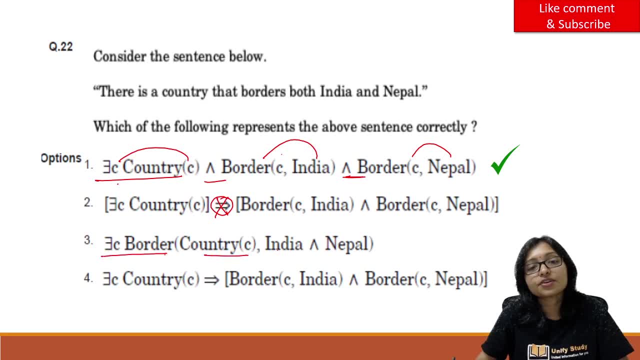 india also. that country is the border of nepal also. india also. that country is the border of nepal also. here it is telling there is c border of country. here it is telling there is c border of country. here it is telling there is c border of country. it's totally a wrong predicate. it is also implies: 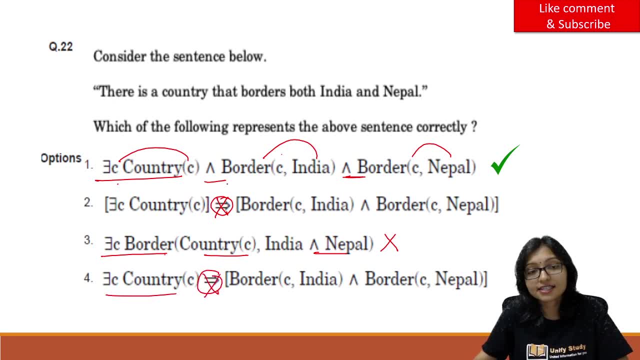 it's totally a wrong predicate. it is also implies: it's totally a wrong predicate. it is also: implies here: implies will be not here. implies will be not here. implies will be not with the: there exist, it is, and so that's. with the: there exist, it is, and so that's. 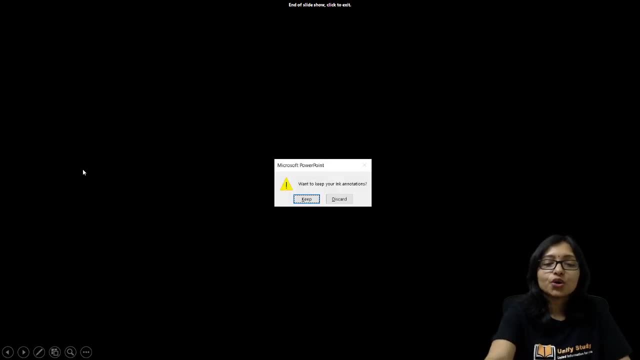 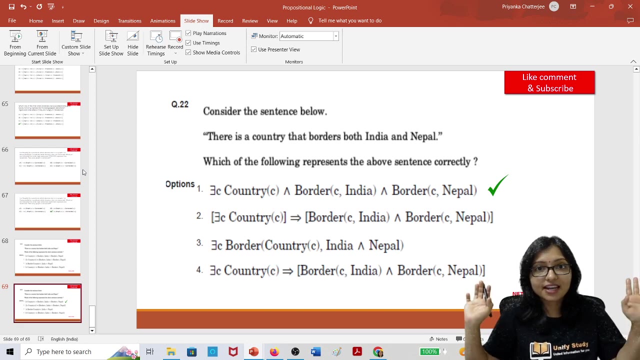 with the there exist, it is, and so that's why this is the answer, why this is the answer, why this is the answer. so it's now, so it's now, so it's now. end of the class. end of the class. end of the class. i hope you understand everything. predicate. 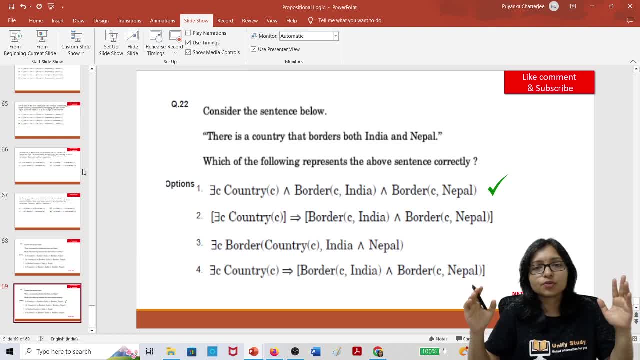 i hope you understand everything predicate. i hope you understand everything predicate: logic, proportional logic. how to solve logic, proportional logic. how to solve logic, proportional logic. how to solve so many questions. we solve there, these so many questions. we solve there, these so many questions we solve there. these are the gate question. ugc net question. 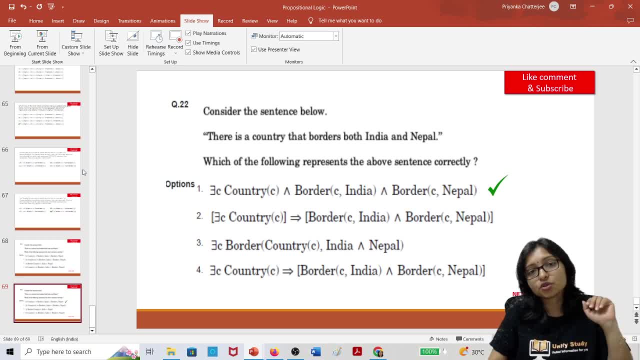 are the gate question. ugc net question. are the gate question- ugc net question. most of them are ugc net questions. some- most of them- are ugc net questions. some- most of them- are ugc net questions. some of them are gate question also, but of them are gate question also but 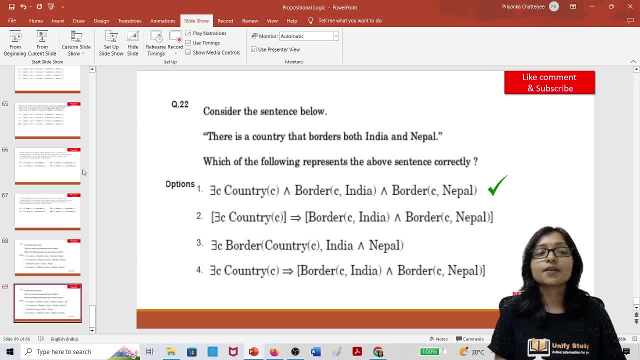 of them are gate question also, but whatever exam it is, but question are whatever exam it is, but question are whatever exam it is, but question are good quality question, good quality question, good quality question and i hope after doing this question and i hope after doing this question, 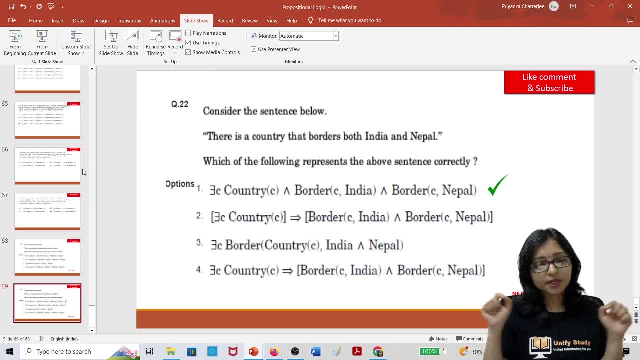 and i hope, after doing this question, your total concept is clear. your total concept is clear. your total concept is clear. so please let me know in the comment. so please let me know in the comment. so please let me know in the comment section and stay tuned with this. 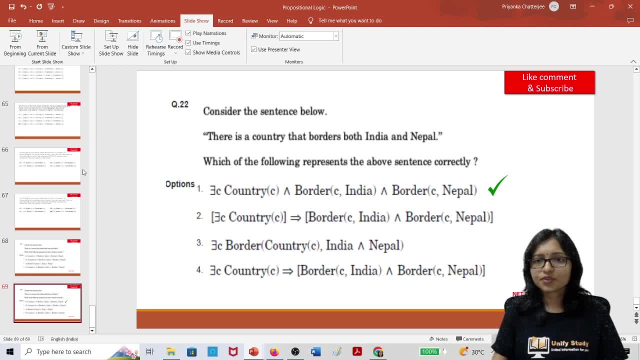 section and stay tuned with this section and stay tuned with this channel, and i hope you did not forgot to channel and i hope you did not forgot to channel and i hope you did not forgot to subscribe, subscribe, subscribe. so definitely subscribe to the channel. so definitely subscribe to the channel.